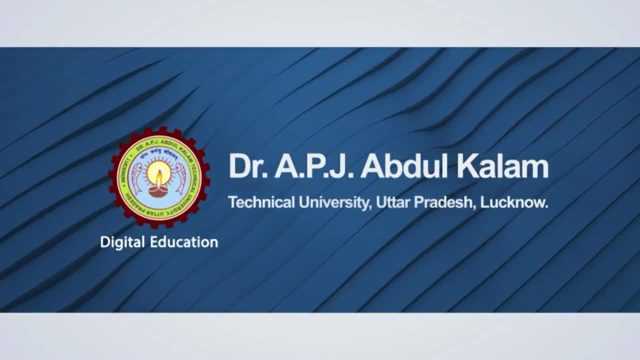 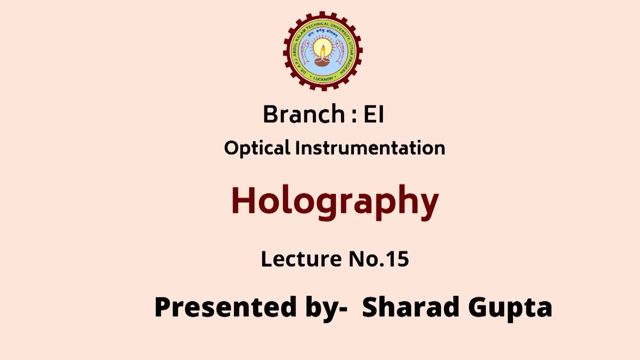 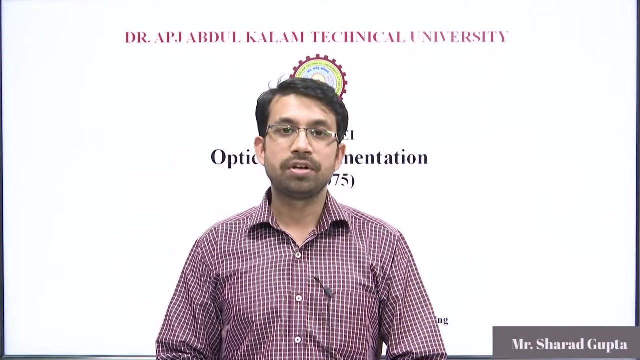 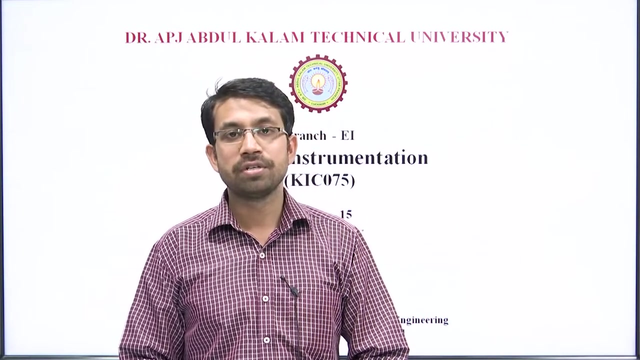 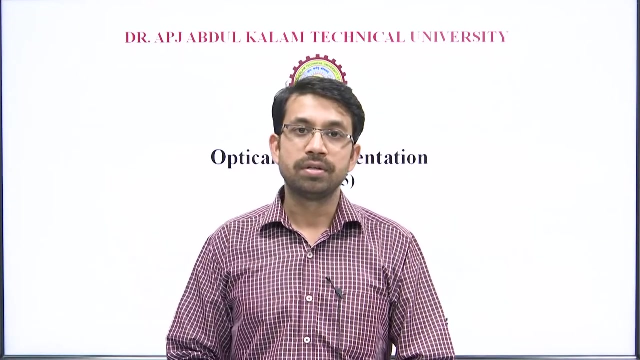 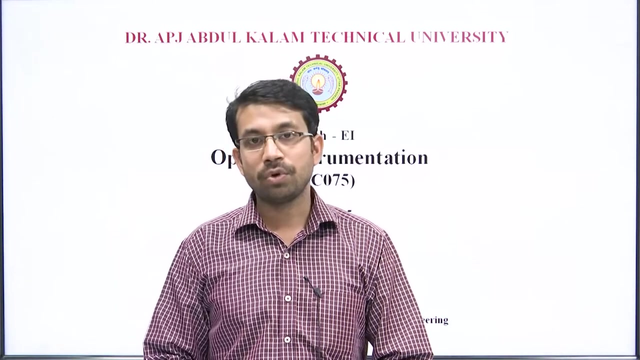 Hello and welcome to the 15th lecture of Optical Instrumentation. My name is Sharad Gupta And so far we have discussed three modules of this subject. Today we shall start fourth unit of this subject and the first part of fourth unit is holography. So what is holography? 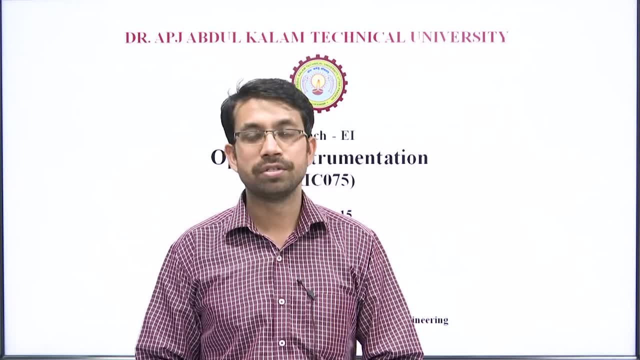 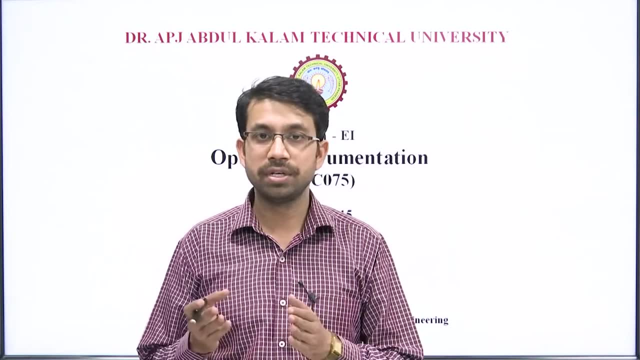 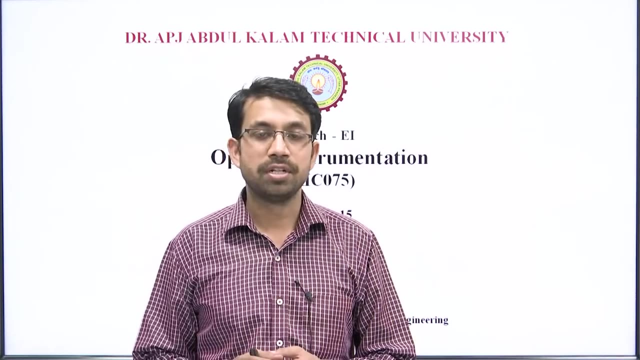 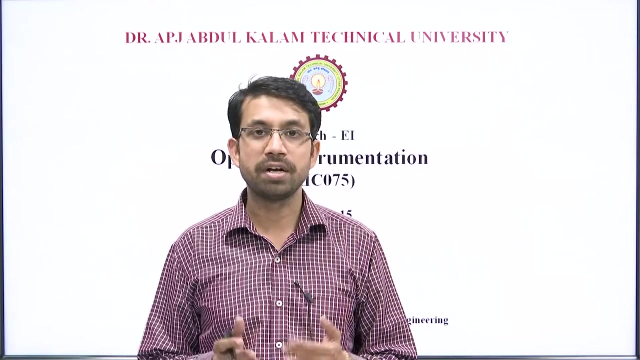 Holography is a method of recording 3D images, The images, the pictures that we capture using normal camera or digital camera or our mobile phone. all these images are in two dimensional. They are called 2D images, Similarly the television that we see at our home or the. 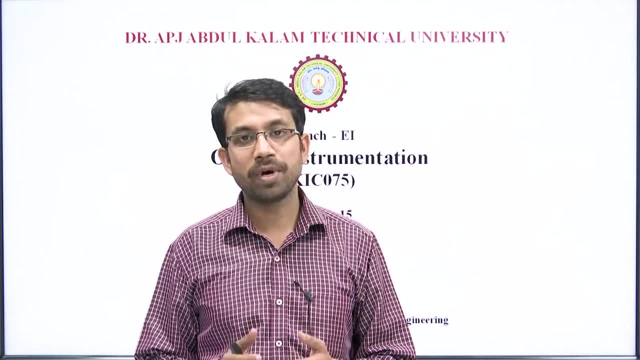 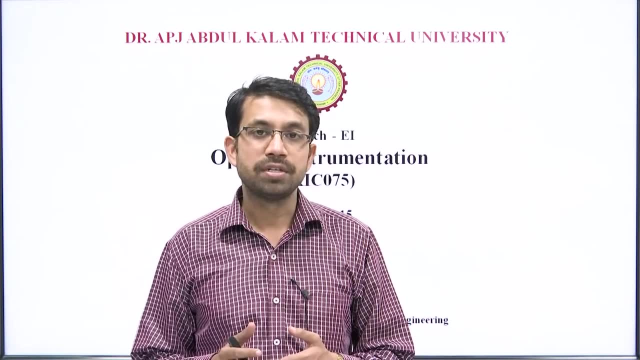 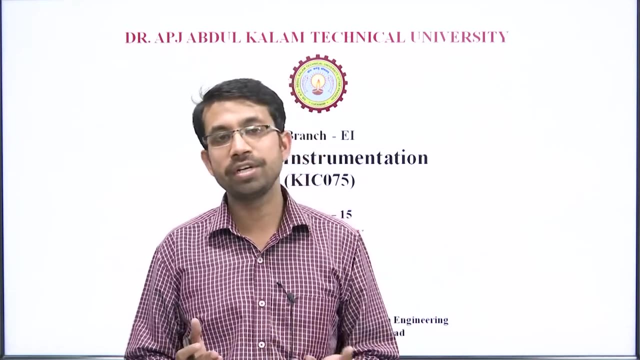 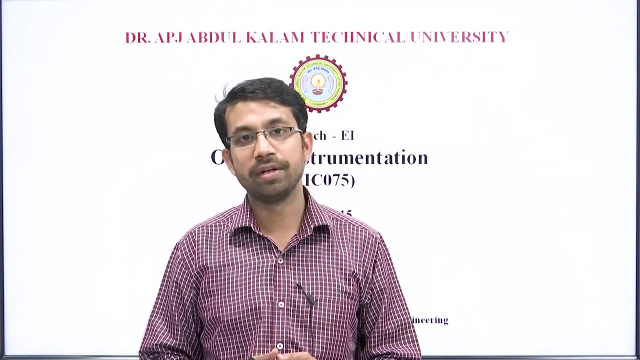 videos that we record using our mobile phones. they all are in 2D Because the images they are two dimensional images. They have x-axis, y-axis, and the information of intensity in two dimensional is recorded either on a photographic film or on a sensor array. These images they do not have the 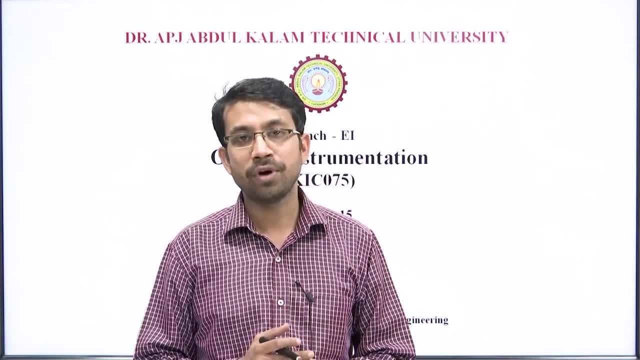 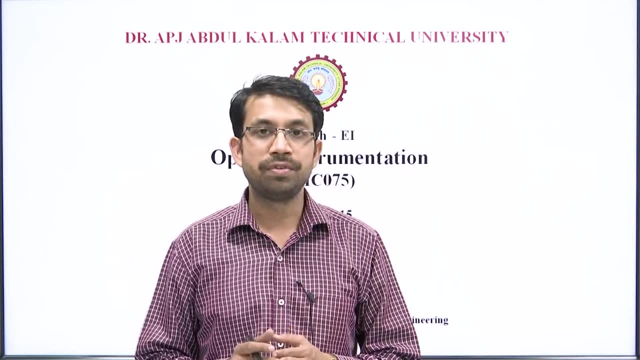 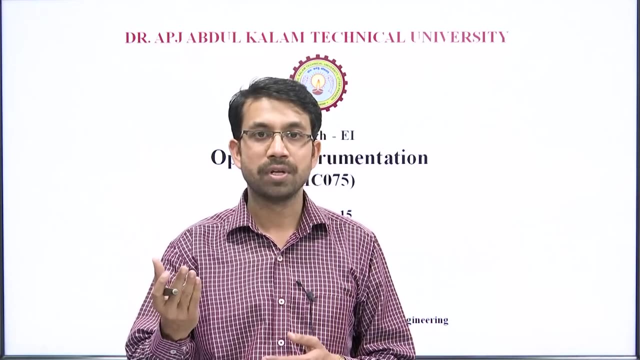 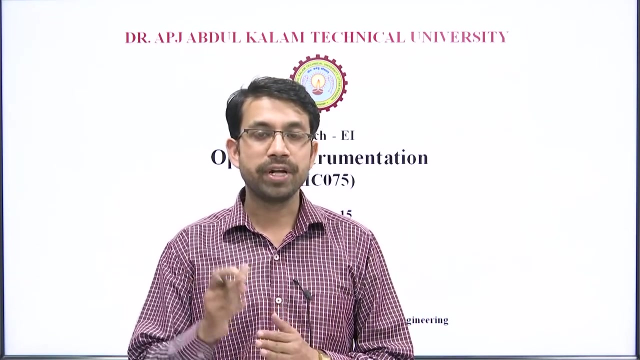 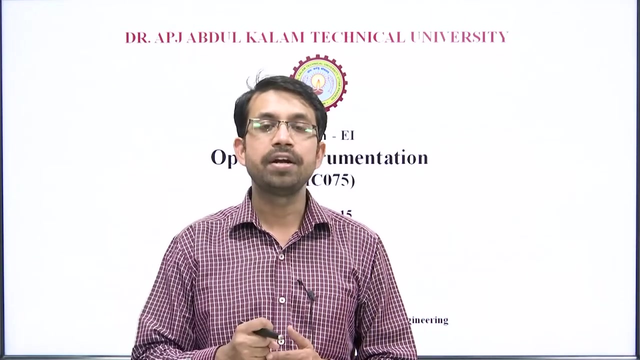 information of depth. While, like our eyes, we can see things in 3D, We can judge which thing is near and which is far Like. if we see a object, we can judge, for example, how a image is recorded, The light that is reflected from any object that reflected light rays. 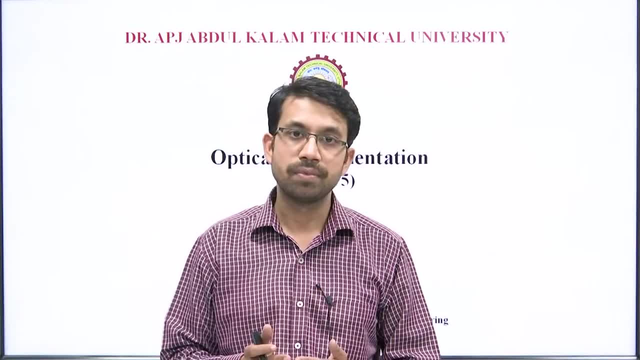 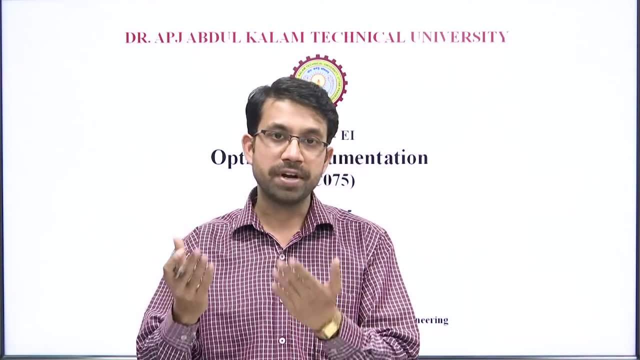 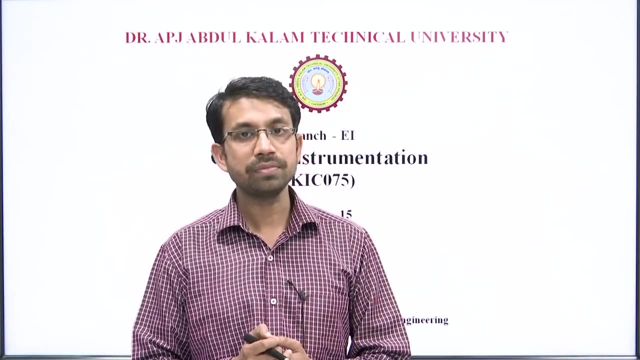 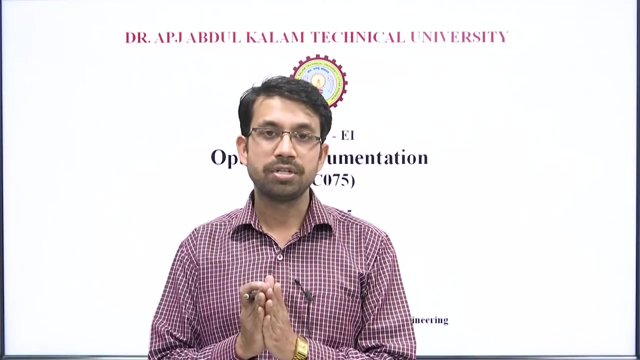 are recorded on any photographic film or on any sensor array and in our eyes, the light rays that are reflected from any object, they are focused on the retina of our eye right. So, this focus of our eyes, they capture the information of intensity and also they capture 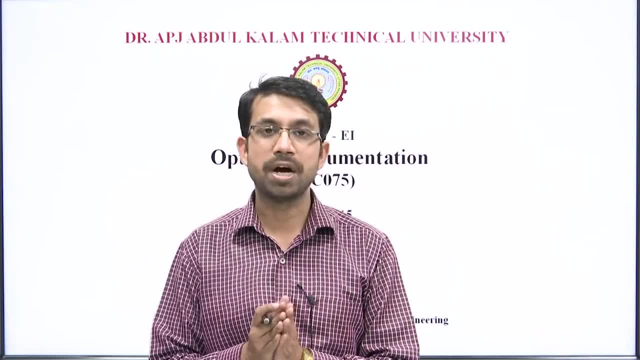 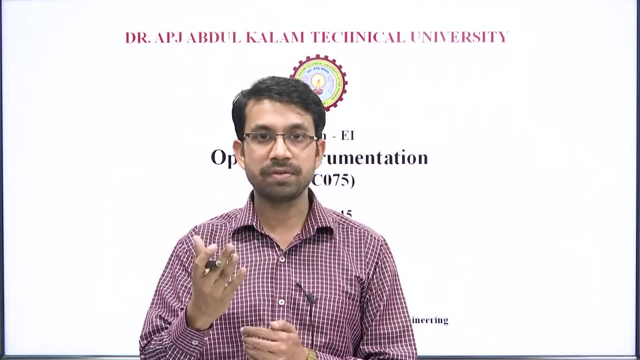 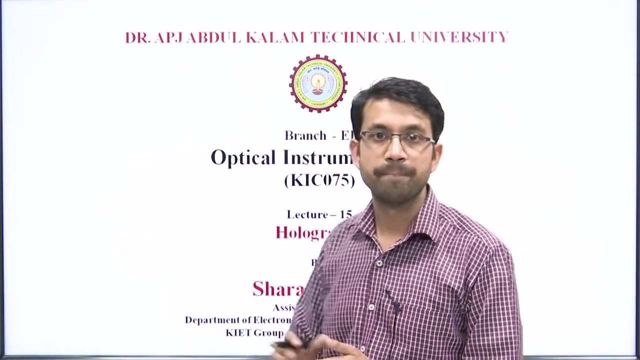 the information of depth or, I must say, path difference. For example, the light ray that are reflected from my face will travel less than the light rays that are reflected from this screen right, So the light rays that are coming from this screen will travel more. 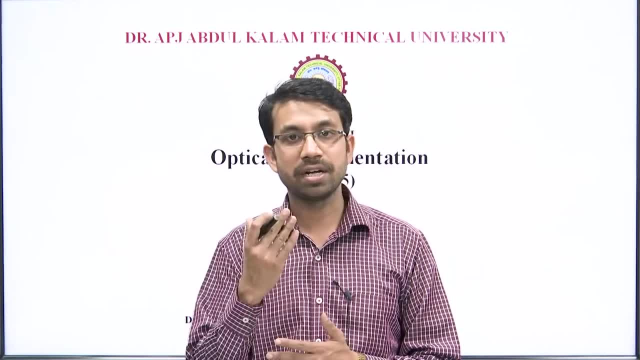 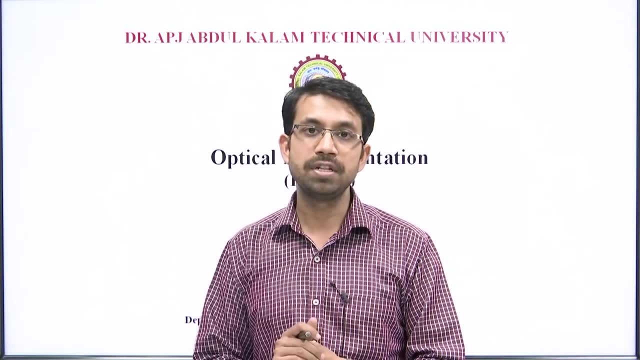 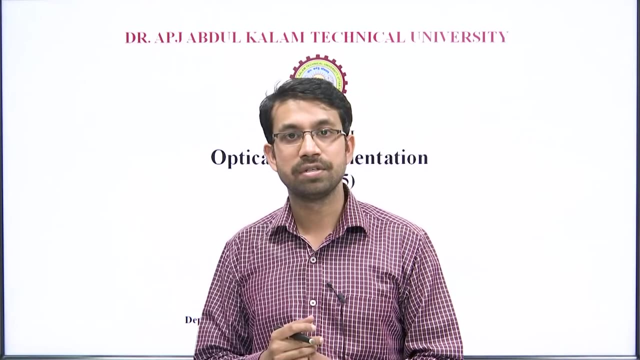 path than the light ray that are that are reflected from my face. okay, So, due to this, there is a path difference between these rays- the rays that are coming from this screen and the rays that are coming from my face. right, Due to this path difference, there is. 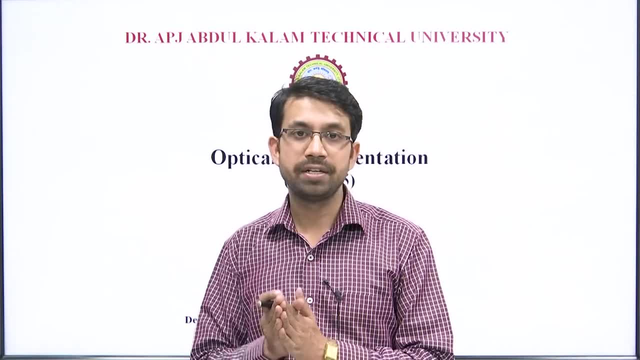 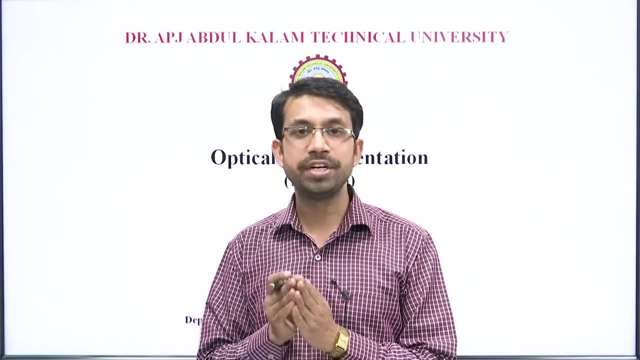 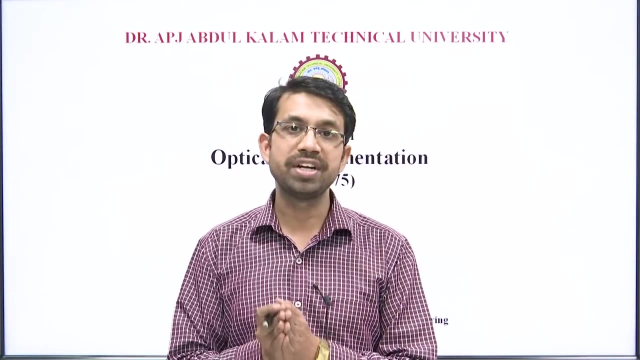 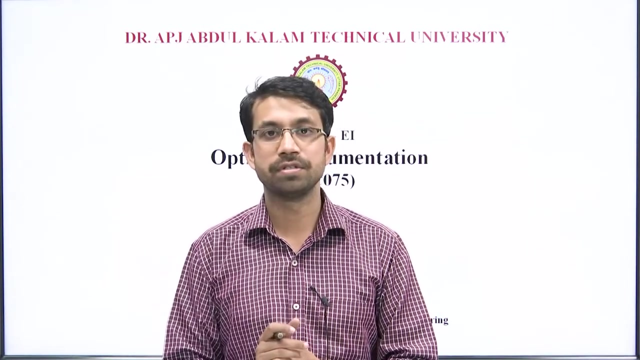 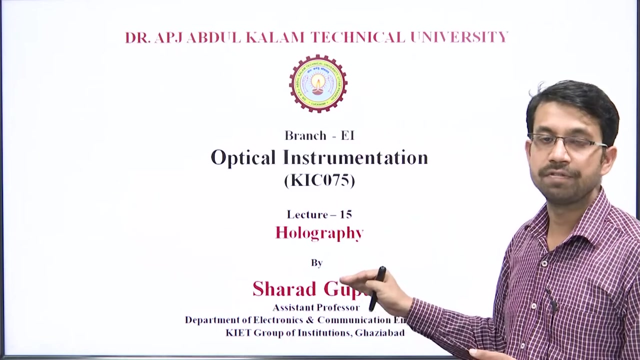 some phase difference and the information of this path difference and phase difference is important to record 3D images, Our normal day to day life cameras. they only record intensity of light. they do not record information of this path difference or phase difference. So this is the method of recording intensity, as well as information of phase difference. 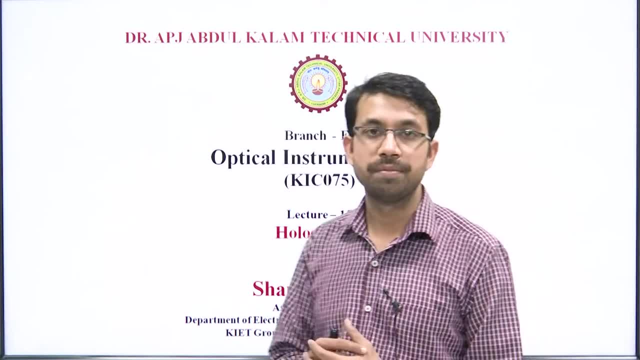 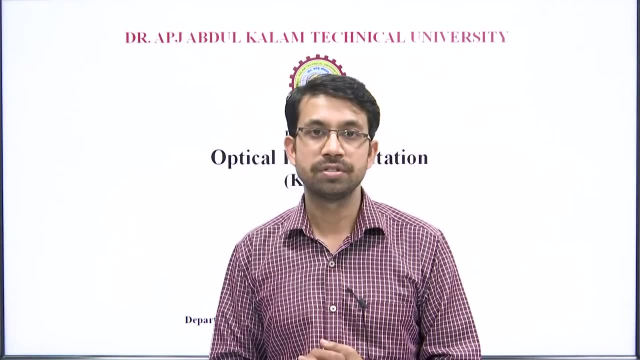 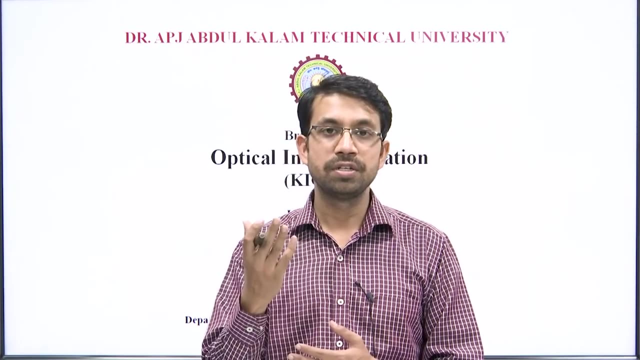 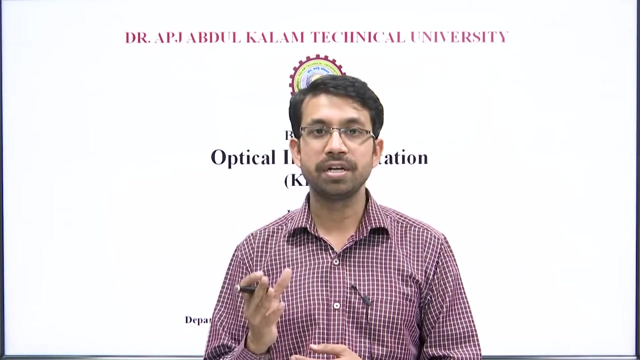 this is called holography, So it is a way of recording, Recording 3D images. you must have seen 3D movies in theatres, So in few scenes of the 3D movie we can see depth, also with intensity, with information of intensity and colour. we 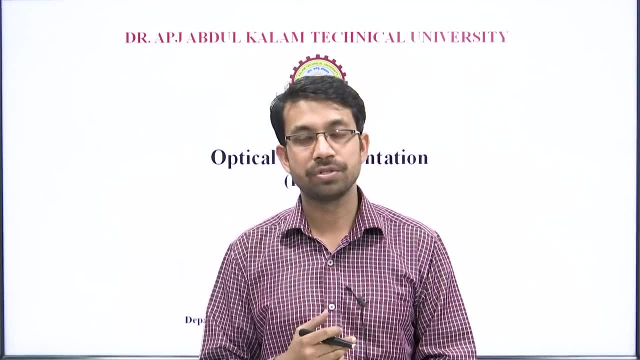 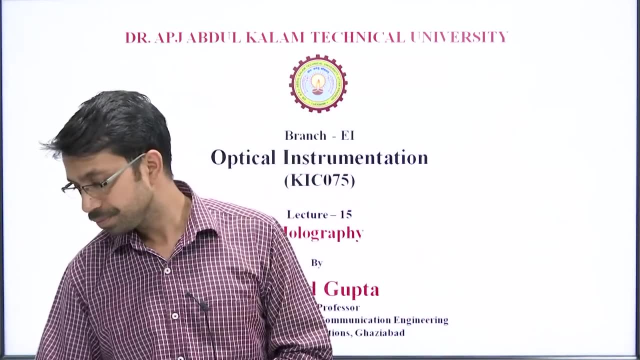 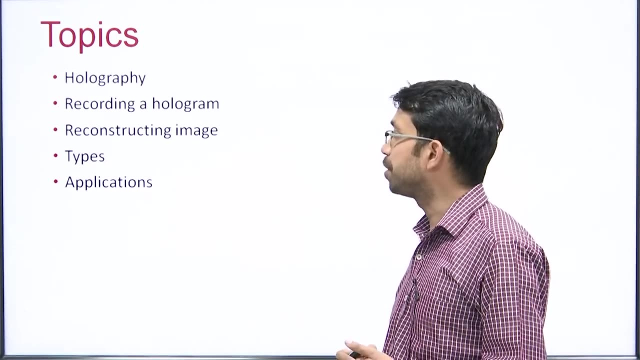 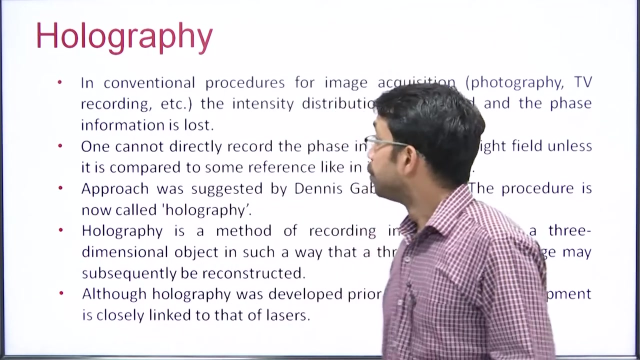 can also. our light can also see depth. So if we can see depth in images, we call them 3D images. okay, So today's topics are holography recording a hologram reconstructing image, its types and its applications. So in conventional procedures for image acquisition, for example, 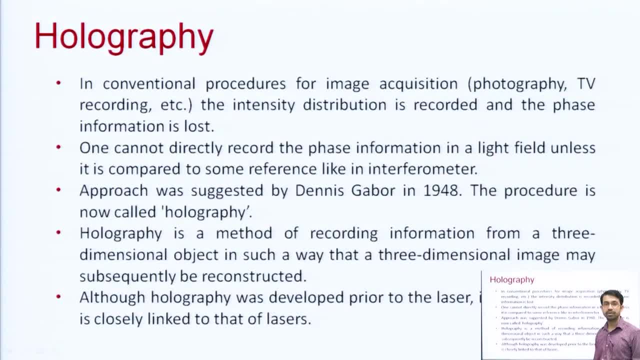 photography, TV recording, etc. either video recording or photography. the intensity distribution is recorded. Only the information of intensity is recorded and phase information is lost. The information of phase is lost, So they are only 2D images. They capture information of intensity and 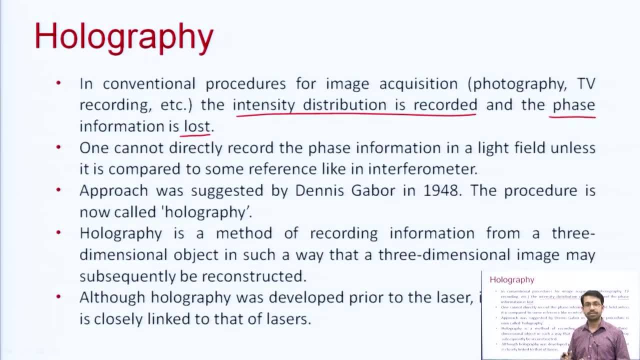 colour in x and y axis but not in z axis. They do not record depth, okay, So this is a way of recording. One cannot directly record phase information in a light field. So it is not easy to record the information of phase unless you compare it with a reference beam or if we compare. 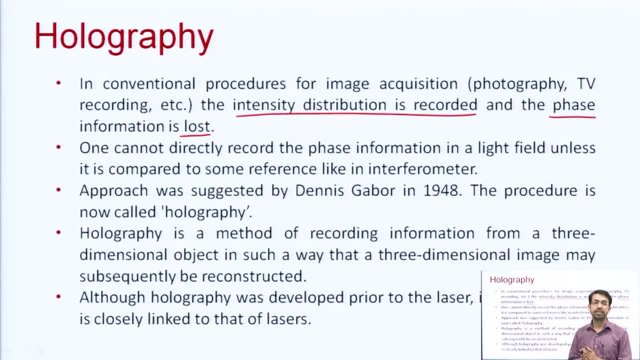 it with a reference beam and then we record it. then it is called a interference pattern. okay, information in a light field, unless it is compared to some reference like in interferometers. In interferometers we have seen in unit number 3 that we divide the monochromatic light into. 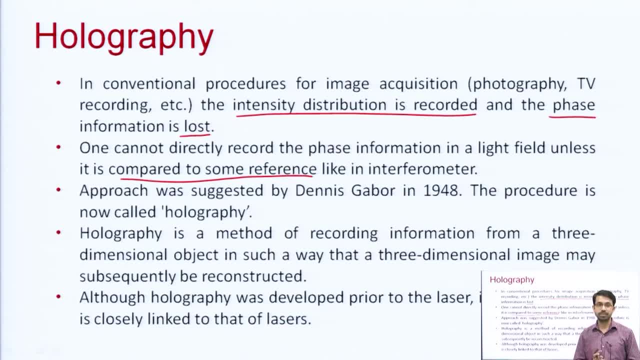 two beams, one is reference and one is test beam, same in spectrophotometers or in Reilly's refractometer. So we have to generate a interference pattern to record the information of phase. ok, So this approach was first suggested by Dennis Gabor in the year 1948 and he called 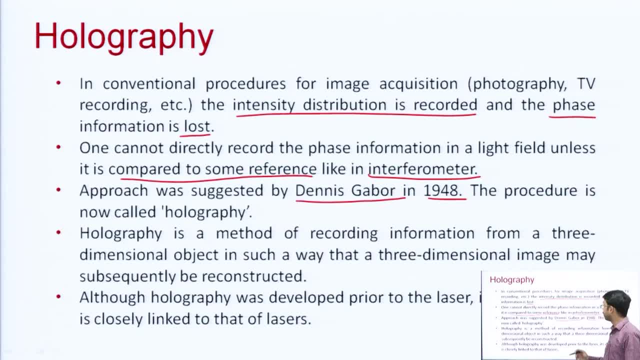 this procedure holography. So who invented holography? Dennis Gabor. It is a method of recording information from a three-dimensional object. So it is not like you can create a 3D image using a 2D image. no, We need actual object for recording. 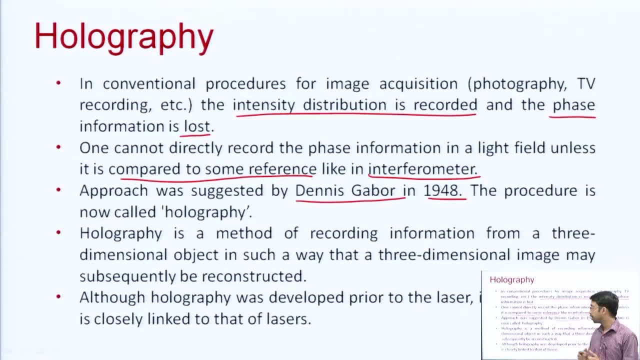 a 3D image for making a hologram. ok, So it is a method of recording information from a three-dimensional object in such a way that three-dimensional image may be subsequent constructed. So the image is recorded in such a way when we reconstruct the image. 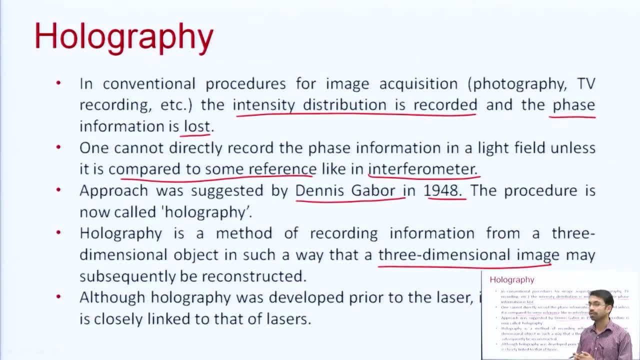 the image feels like a 3D object. ok, Although holography was invented before the invention of laser, but because highly monochromatics light source is required to record holograms, So theseALLT is closely linked with the development of lasers. So as better lasers. 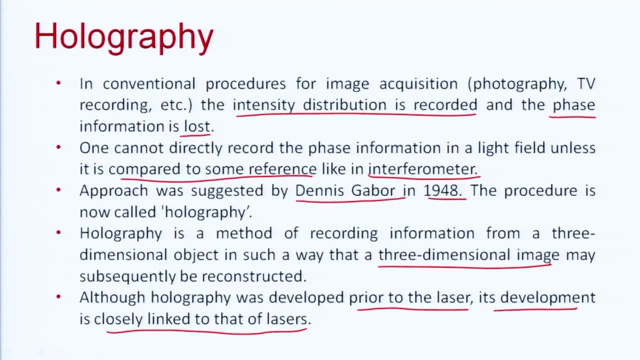 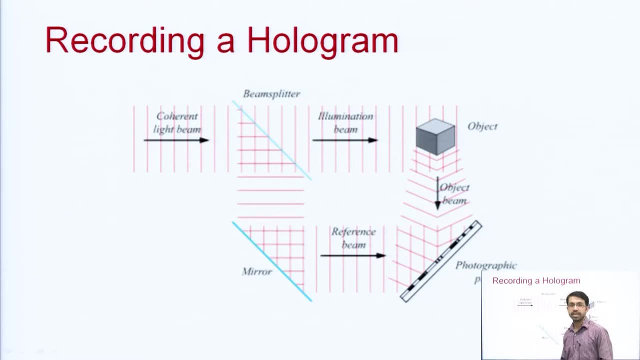 came into market. as more research was done on laser and better and better lasers were manufactured, also better holograms were easily made and recorded. ok, So this is the image that explains the process of recording a hologram const. So, as you can see, there is a coherent light wave front that is coming from this direction. 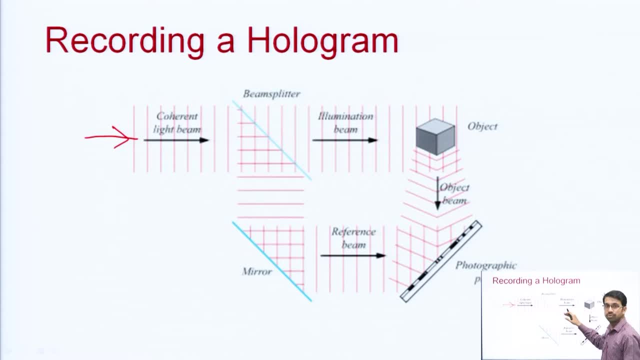 This is a beam splitter. it is dividing this wave front into 2 parts. it is capped 45 degree from the incoming beam, So half part goes here, half part goes there. this is the 3D object for which we have to record a hologram. we have to record 3D image. So this is just 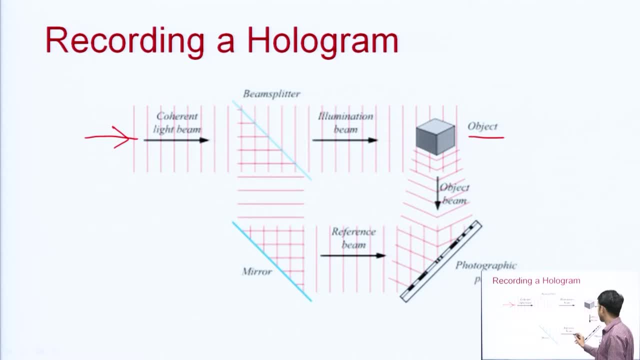 reference beam. this is mirror, it is reflecting the reference beam and also this is the object. this object is illuminated using this coherent light beam, So it will reflect light from its different, different surfaces and accordingly, this wave front will be converted like this: ok, So this is the wave front and this is the reference. 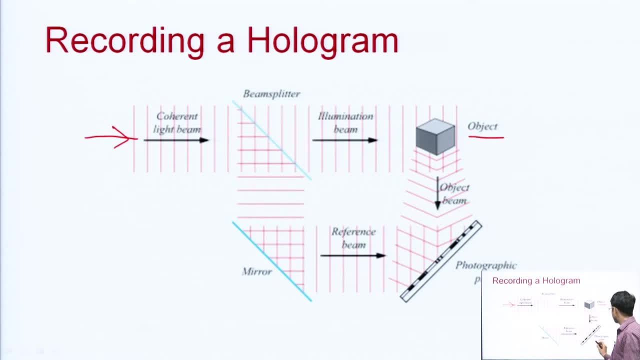 beam. this is called object beam, So they will illuminate this photographic plate or a sensor array, right So photographic plate. what we will get on this photographic plate? we will get a interference pattern, Interference of this reference beam and this object beam. So this will have information. 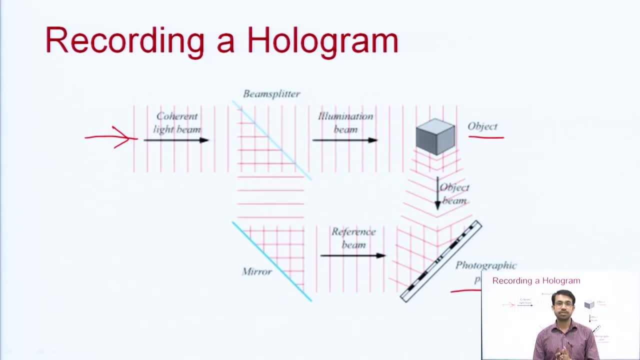 of intensity and also it will have information of phase difference or path difference. why? because this is interference pattern and this wave front is modified like this and so So It is compared with this reference beam, So we get interference pattern. So this is a 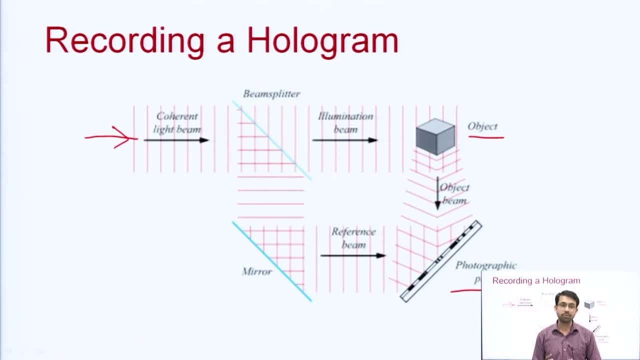 hologram. Now we have recorded a hologram, How do we see that the image is 3D or 2D? So we have to again illuminate this photographic film using the same wavelength of light, using a coherence or same coherent light source of same wavelength We have to illuminate. 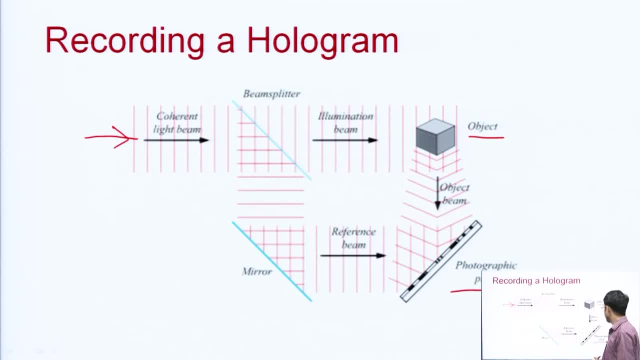 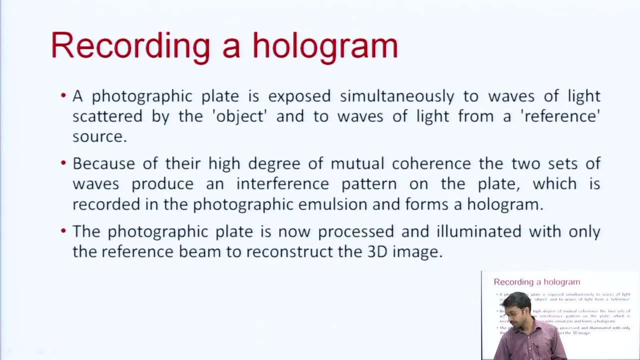 this reference beam and when we do this viewer over here will feel that there is a 3D object kept here. So how do we record a hologram? A photographic plate is exposed simultaneously to waves of light scattered by the object And to the waves of light from reference. So object beam and reference beam So simultaneously. 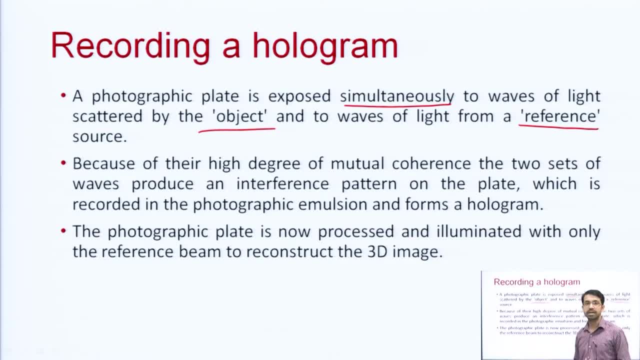 we are exposing a photographic plate, So what we will get? We will get a interference pattern. Because of their high degree of mutual coherence, the two sets of waves produce an interference pattern on the plate right, which is recorded in the photographic emulsion. 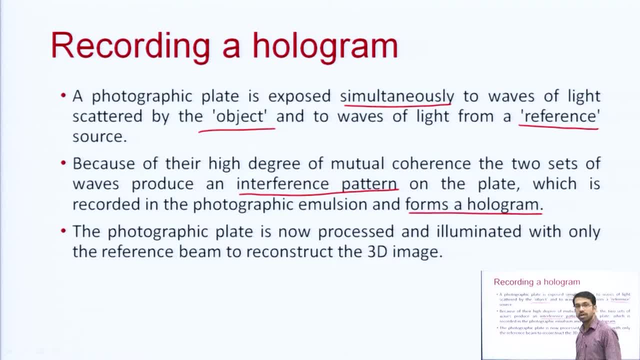 and forms A hologram. What is what do we call a image that is created using holography, A hologram? You must have seen holograms on books, on products and a lot of things. The photographic film is now processed and illuminated with only the reference beam to reconstruct the 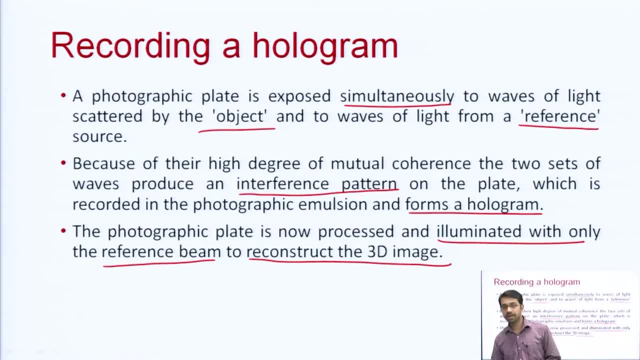 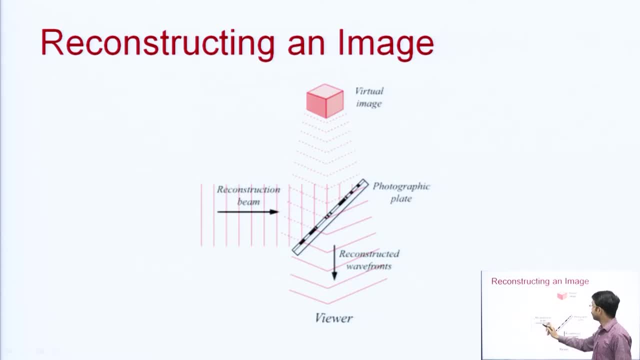 3D image. So let us look at the diagram Over here. So rest of the part is removed, The object is removed. We are, we are illuminating the hologram with the reference beam And what happens? This, this interference pattern. 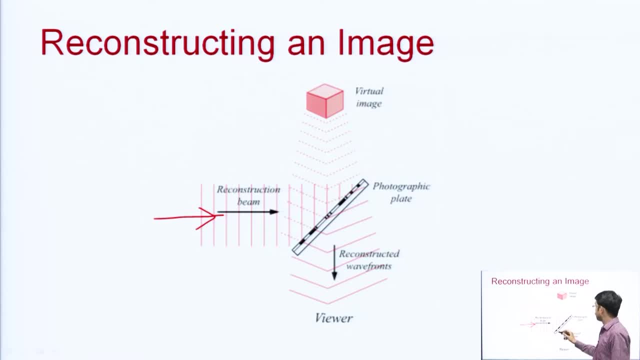 will diffract the incoming light beam in such a way that a viewer, if he is viewing the hologram from here, it seems like there is a actual object kept here. So to his eyes he will feel he will. he will look at a 3D image that that looks like exact object. 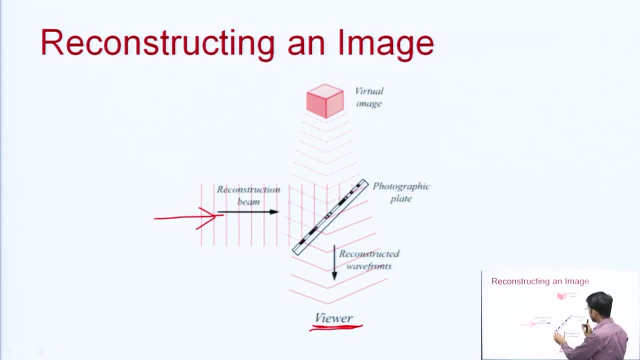 And if, if he moves this photographic plate or I can say hologram, then this 3G, 3D object will also move. If you take a simple photograph in your hand or if you take a mobile camera, if you take a mobile phone and you you view a photo, if you move your phone or photo, like 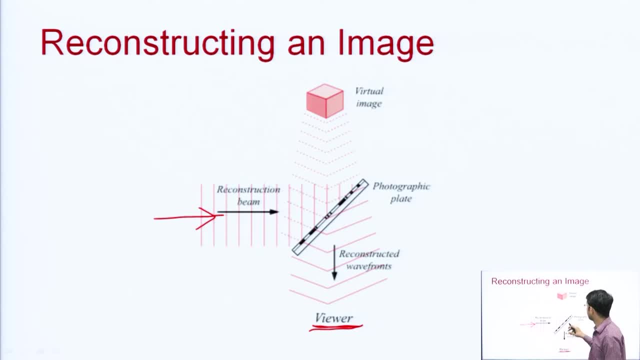 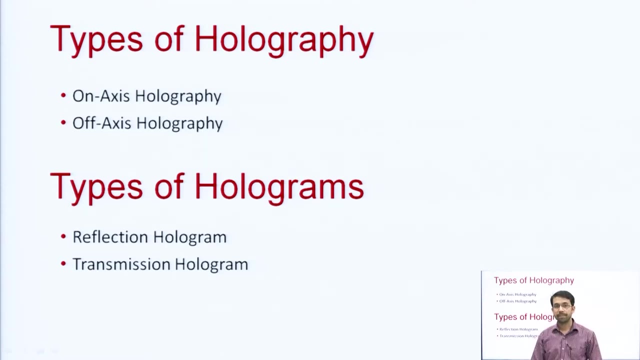 this. it does not move, So it is a 2D image, But if you move this photographic film, this image will move. So this was about how to record a hologram and how to reconstruct image using a hologram. 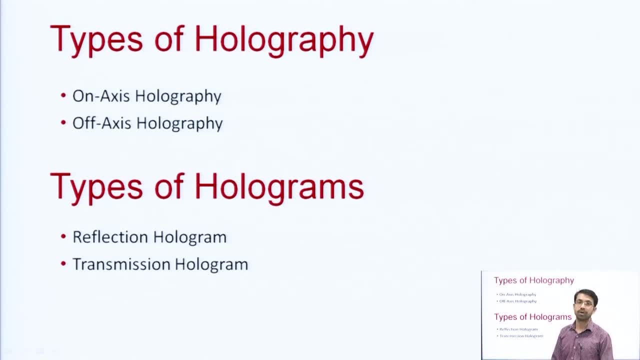 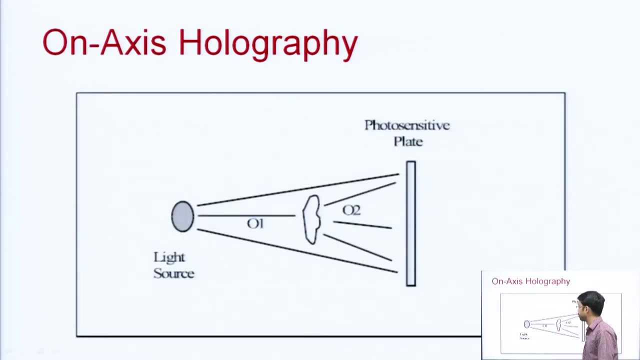 Now next is: what are the types of holography or holograms? One way is to classify the way of recording hologram: on axis and off-axis holography And types of holograms: reflection and transmission holograms, So on-axis holography, If reference beam and object beam, the beam that is coming from. 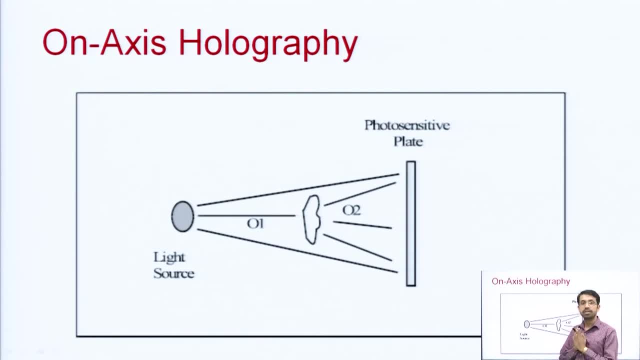 source beam that is coming from the object. they are coaxial. then this method is called on excess holography. So, as you can see, this is monochromatic light source. the reference beam is coming on the photosensitive plate and this is the object for which we have to. 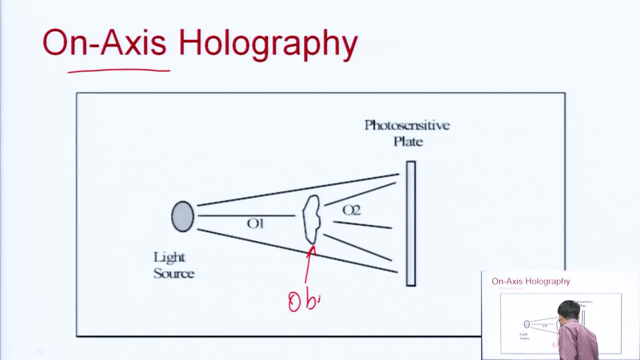 record the hologram object. So the light that is coming from the object that is O 2 is object beam, So they are both coaxial. there is no, there is 0 degree angle between these two beams, So it is called on excess holography. This method is generally. 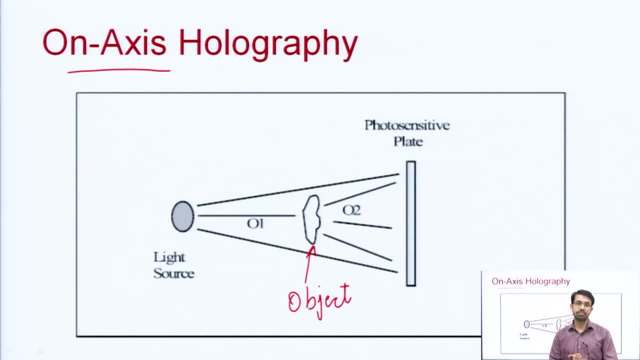 used for a semi-transparent object, or you can say the objects that are non-transparent are not opaque. ok, So this method of recording hologram can be used for semi-transparent objects, and the first hologram that was recorded by Dennis Gabor was on excess was recorded using 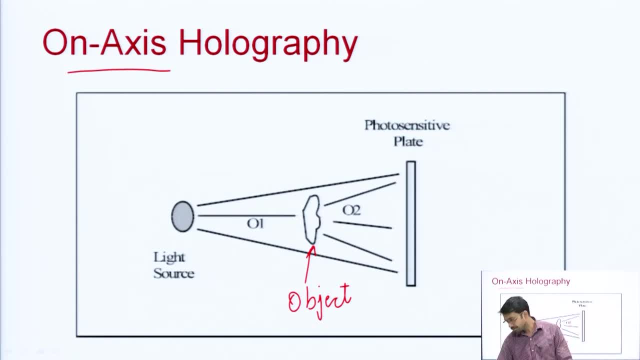 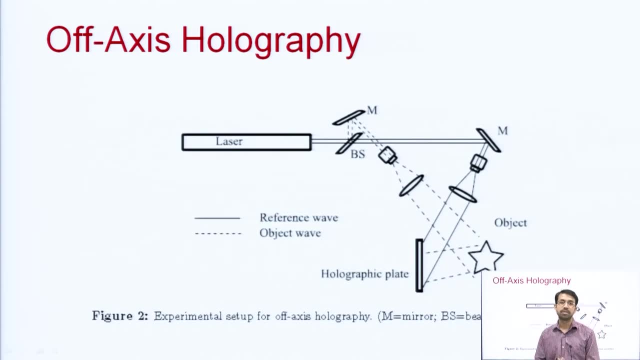 this method on excess holography. Next is off excess holography. If there is a certain angle between reference beam and object beam, then this method is called off excess holography. So look at this diagram. this is a monochromatic light source- laser. ok, This is a beam splitter. 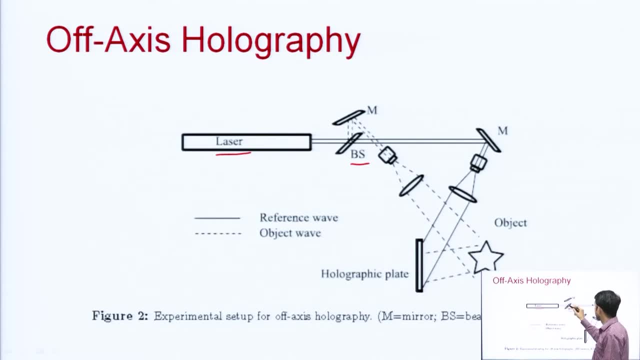 beam splitter is divided into two parts, So half goes in this direction, half goes in this direction. this is a mirror. again, it is reflected by the mirror And this is a lens, collimating lens. it is sorry, this is beam, this is. this is divergent. 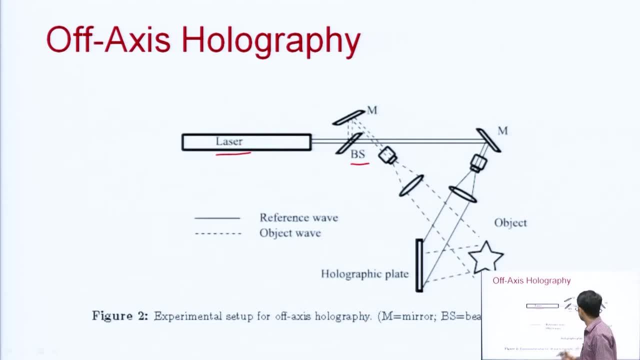 I think also this is miscellaneous, this is a clap, this is collimating lens, So these, So this is diverging the beam and this is collimating the beam. So we are, we are spreading the light. So now this is a parallel wave front coming in this direction and over here. 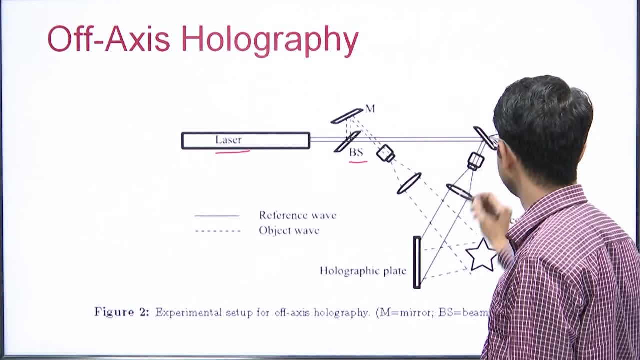 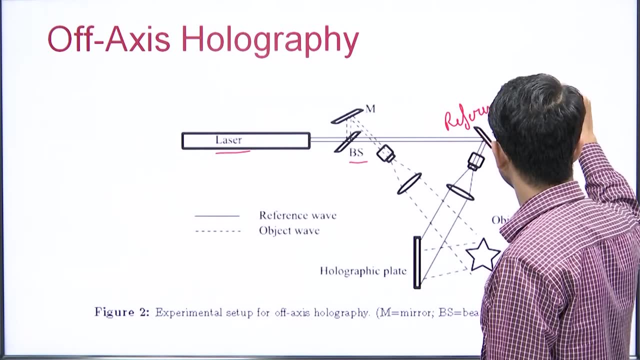 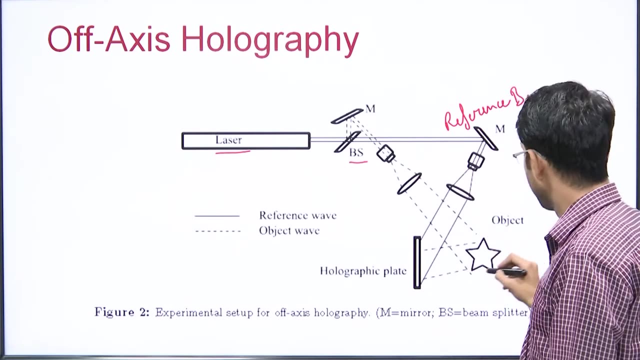 again, this is a parallel wave front. So this is our reference beam, this is reference beam and this is object beam. as you can see, the light is going at the object, it is illuminating the object And now the light rays that are reflected. 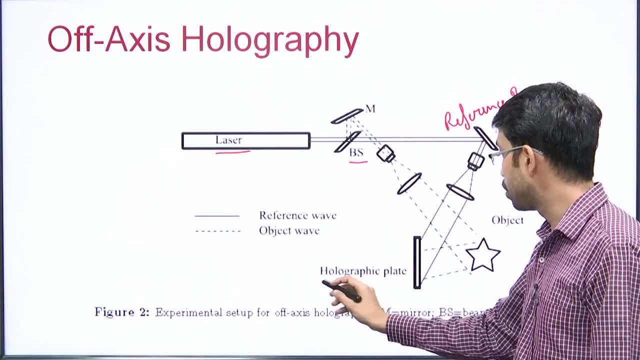 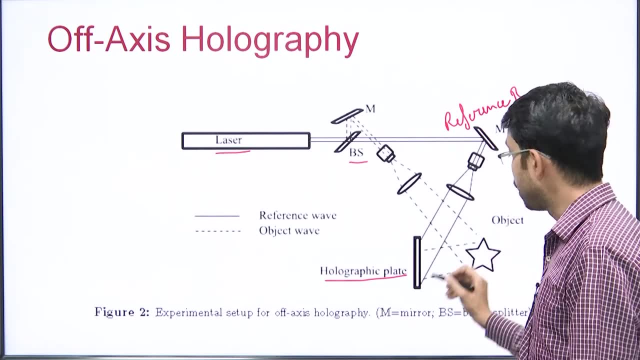 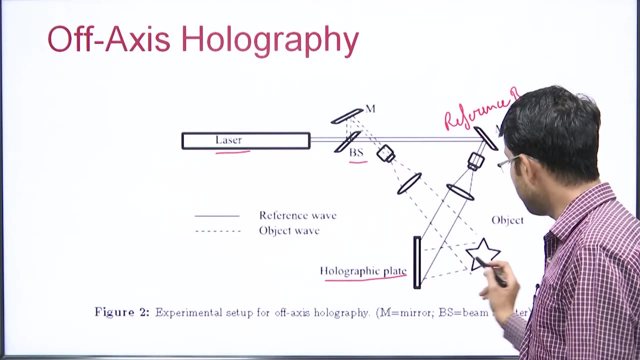 from the object are falling on this holographic plate and this is over. here reference beam is coming. this is object beam, So a interference pattern is recorded on this beam. as you can see, there is a certain angle between reference beam and object beam, So this is called a. 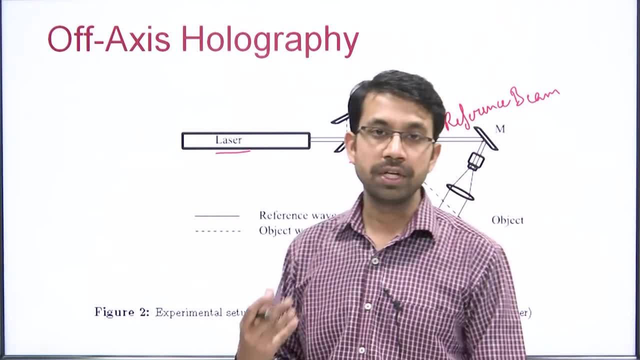 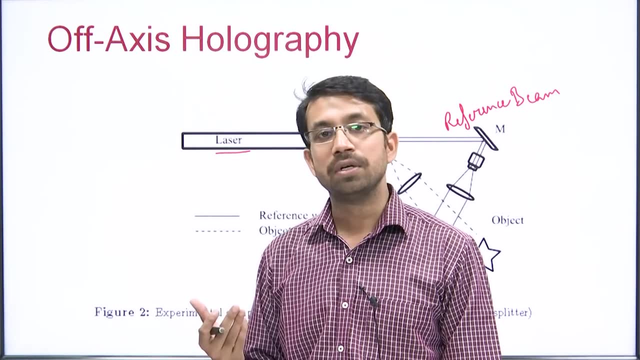 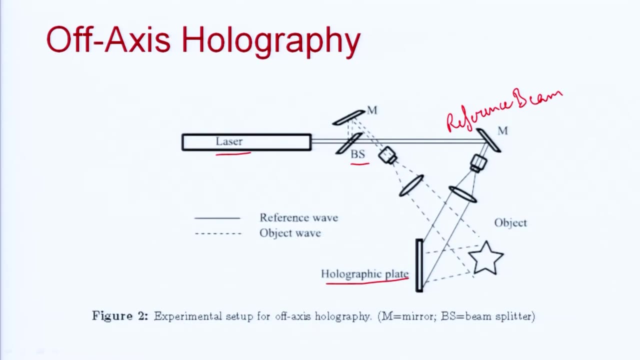 off-axis holography. Normally this method is used for recording holograms, because we can record holograms of opaque objects also. So this is off-axis holography and that was on-axis holography. Remember, if reference beam and object beam are making a certain angle, then it is called 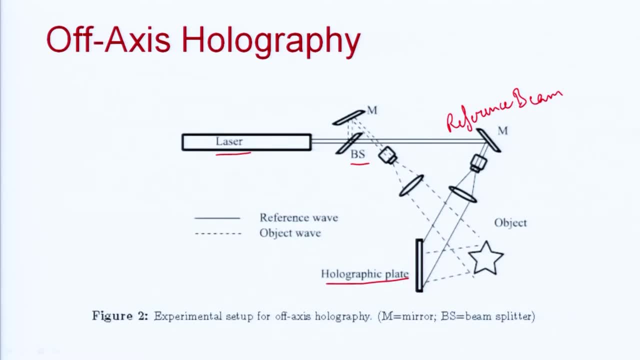 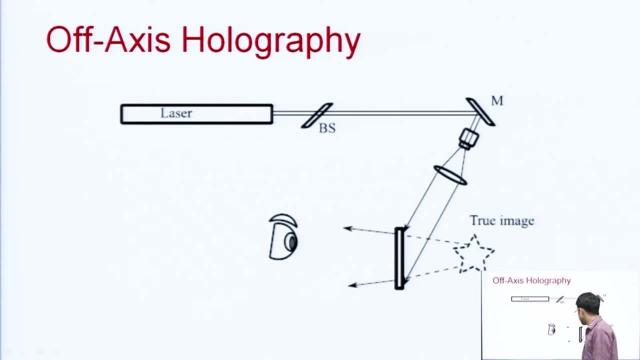 off axis holography, 15. 26. and if they are coaxial, then it is called on axis holography. And this is how we see the image. we reconstruct the image using same reference beam. as you can see, This is the reference beam, this is the image, this is the holographic plate. 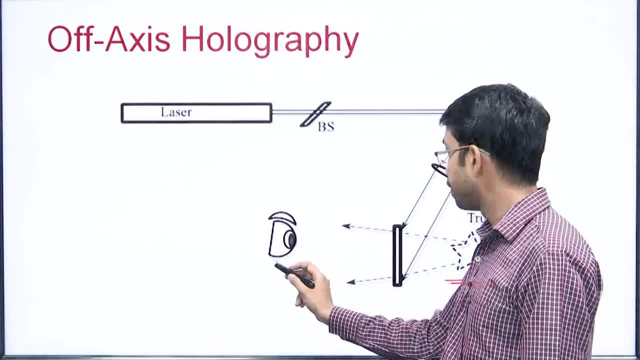 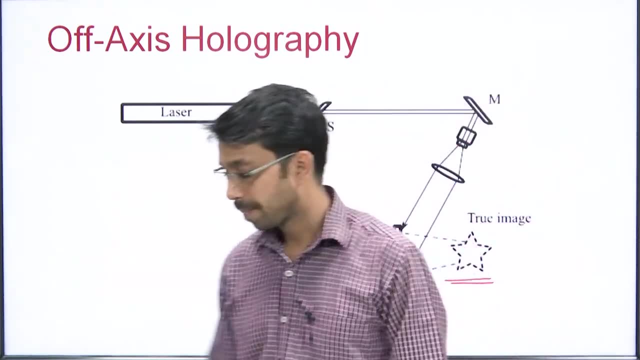 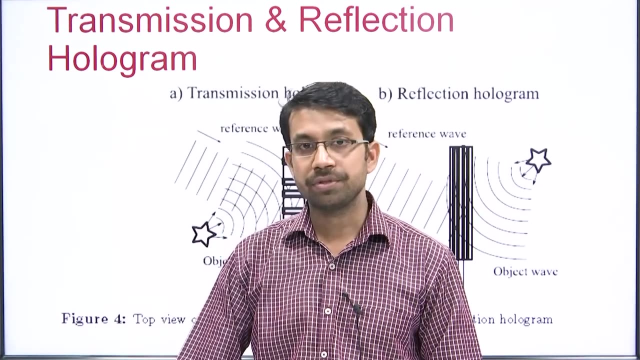 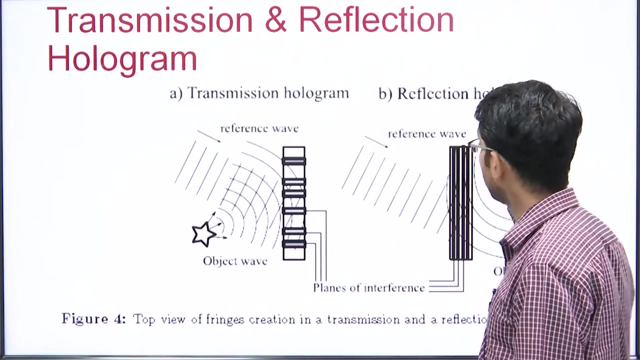 on which image is recorded and if, for the viewer, he will see a image that will feel like a real object. ok, Next, transmission and reflection holograms. ok, So, as you can see, the method of recording a transmission hologram and reflection hologram are shown in this diagram. If we are illuminating, 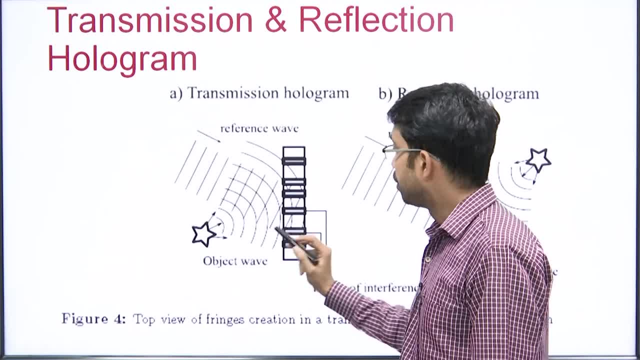 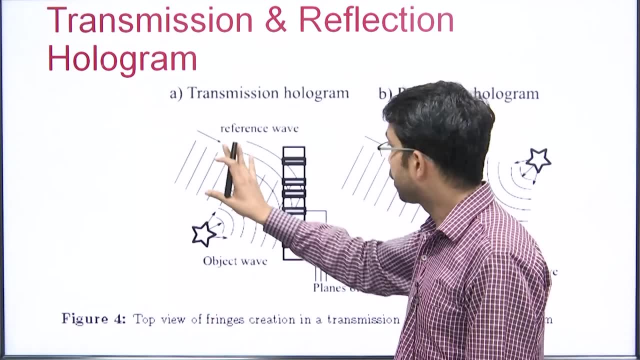 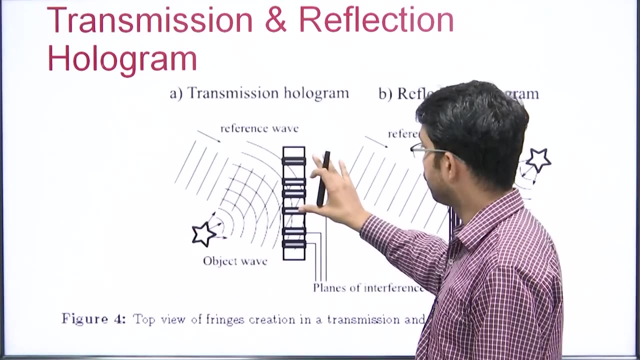 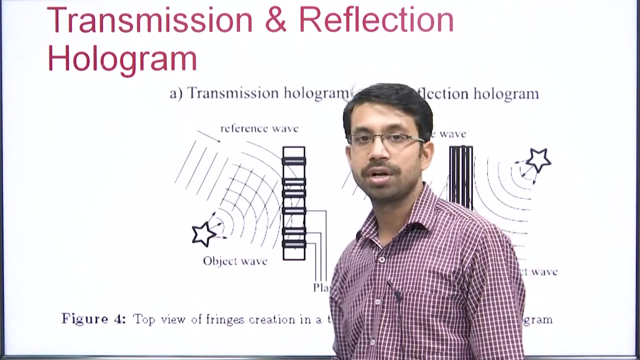 the photographic plate such that the object wave and the reference wave, They are on the same side. the object wave is coming from this direction and, sorry, reference beam is coming from this direction. object beam is coming from this direction. ok, So they are on the same side. So the hologram that we get in this condition is called transmission. 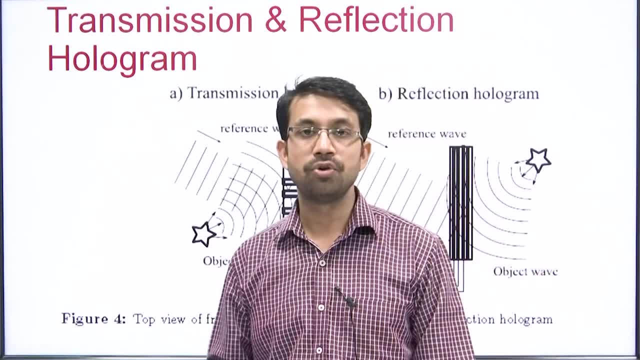 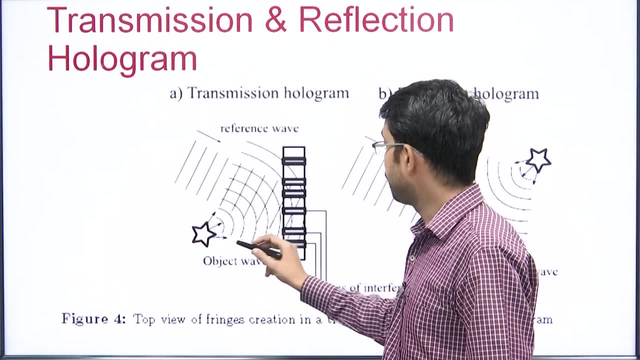 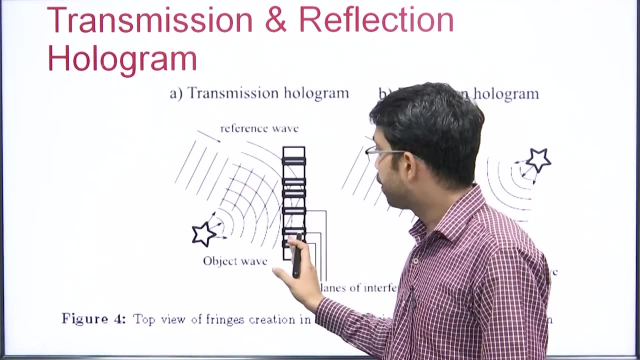 hologram transmission hologram. So, as you can see, this is a method of off axis holography, because there is a angle between reference beam and object beam And also both the beams are illuminating the photographic plate from the same direction. 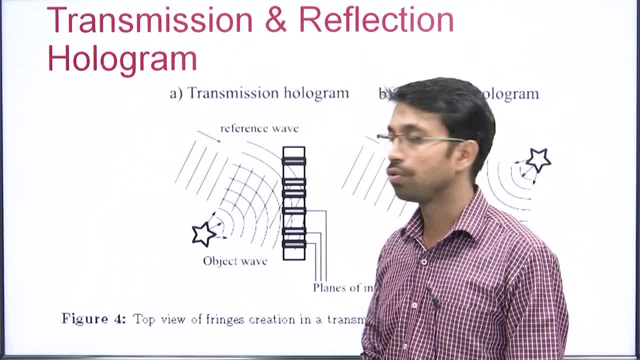 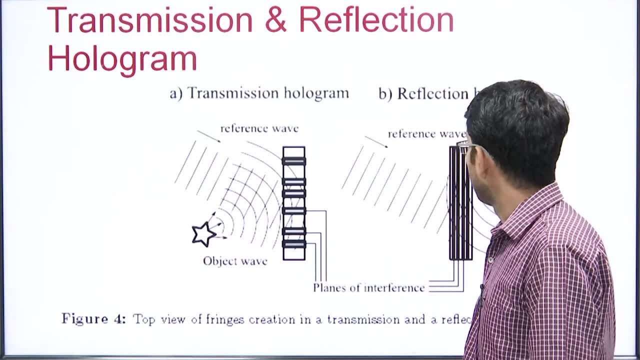 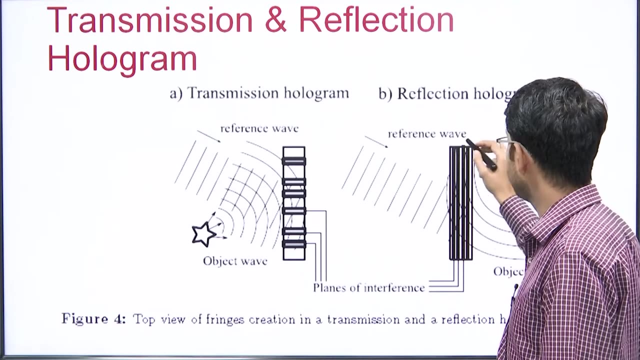 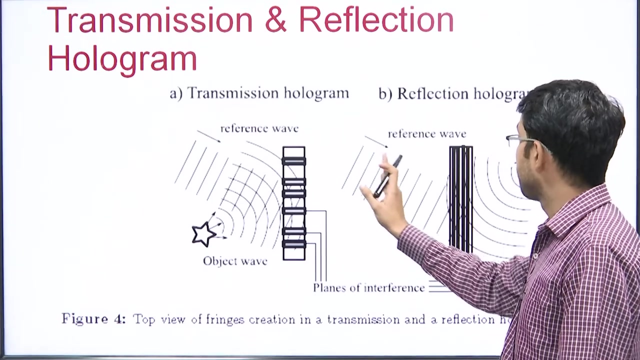 So this method records transmission holograms and the interference pattern. you can see the lines will be drawn like this. On the other hand, how reflection hologram is recorded like this, If photographic plate is illuminated such that photographic film is illuminated like this, So you can see that the reference beam and object beam, they are falling on the 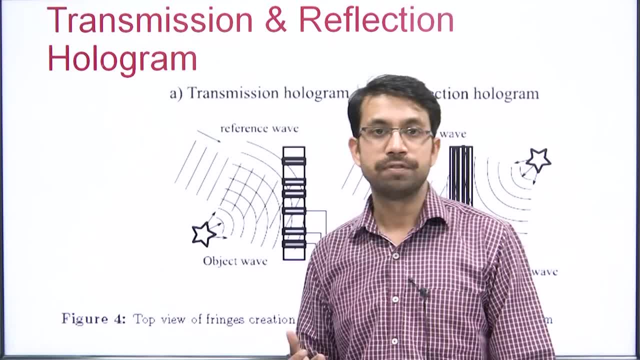 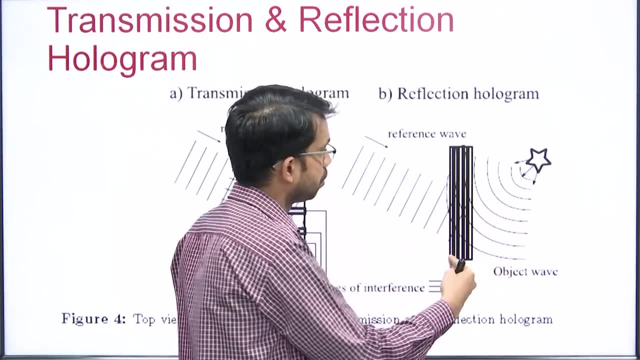 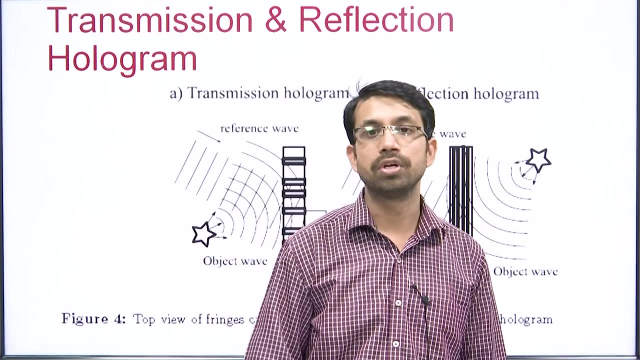 photographic film from opposite directions. from opposite directions, As you can see: reference beam is coming from this direction, object beam is coming from this direction. ok, So in this condition, the hologram that we get is called reflection hologram. What does it called? It is called reflection hologram. 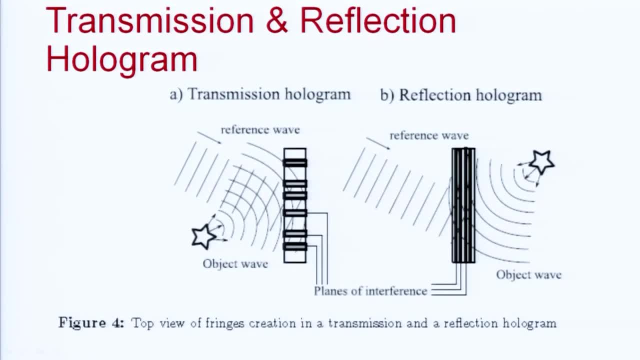 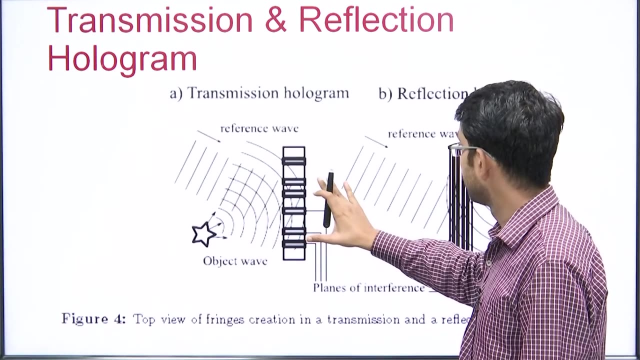 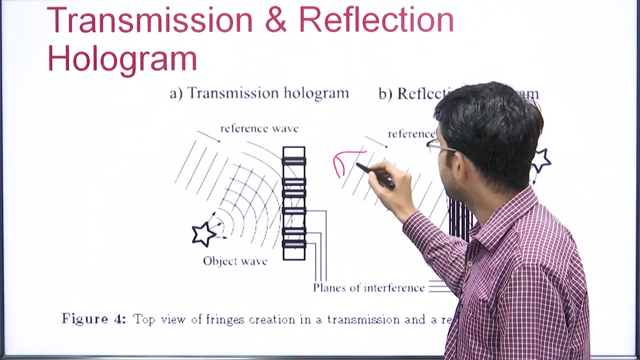 When we are using a transmission hologram, viewer has. if viewer has a transmission hologram, then reference beam has to fall from this direction and viewer will see from this direction Where is viewer In case of transmission hologram. viewer is here here. 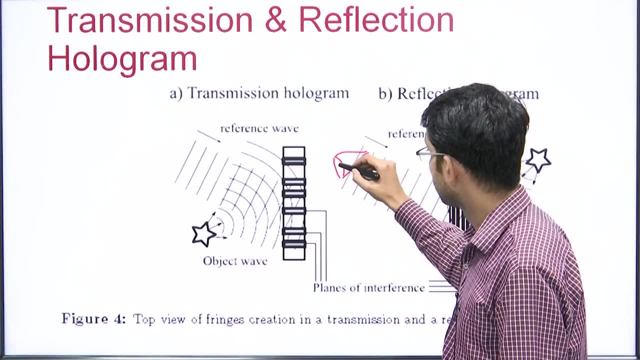 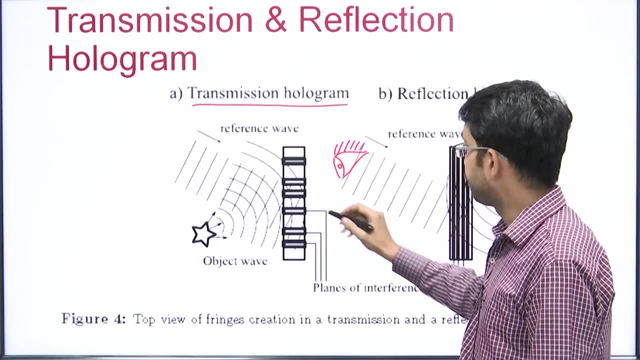 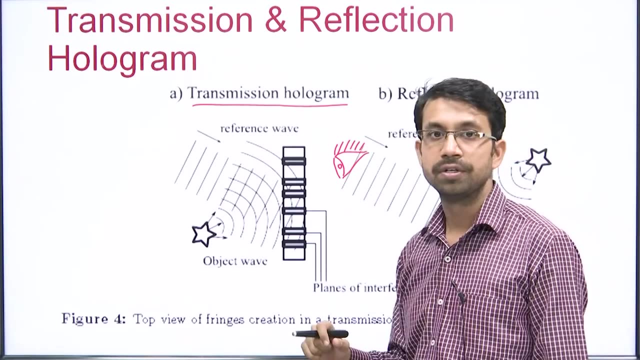 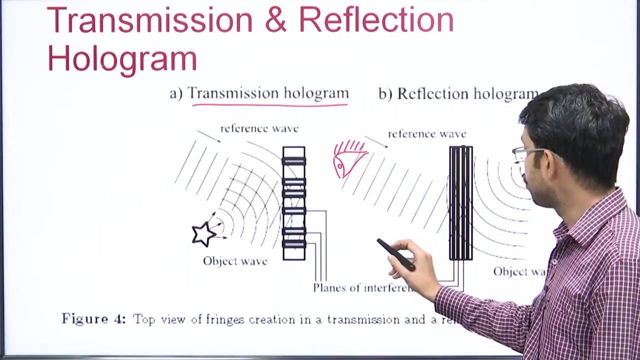 Ok In case of transmission hologram. So if we illuminate this photographic film with the reference beam, viewer will see 3D image from this direction, ok, While in case of reflection hologram viewer has to be over here. 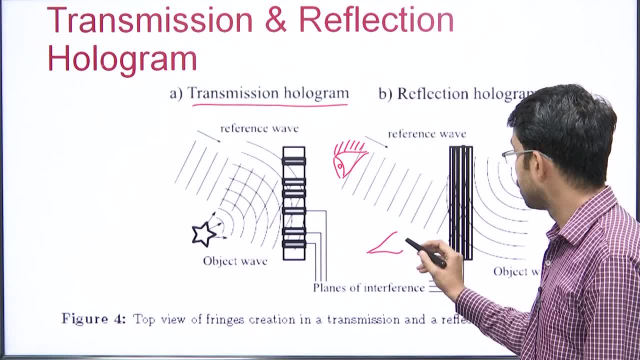 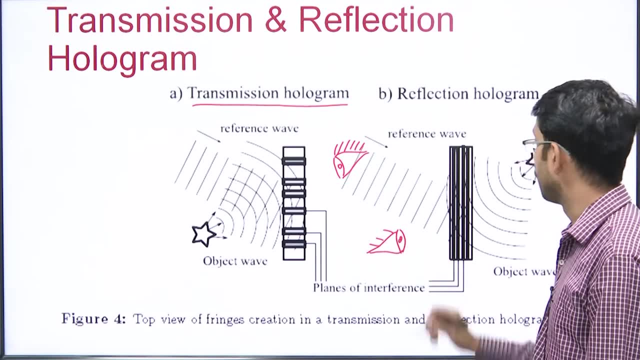 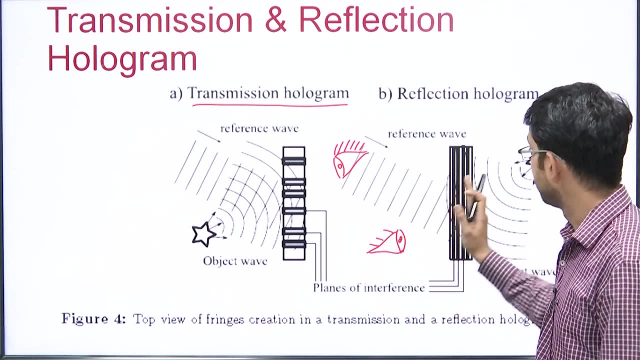 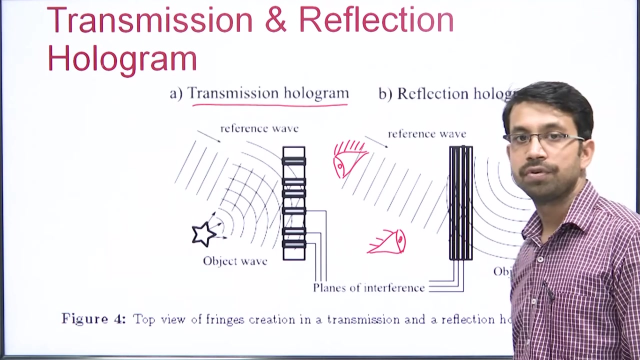 This is the viewer, So reference beam is coming from this direction. it will get reflected from this interference pattern and viewer will see three day image over here on this photographic film. So in this case viewer is on the opposite. 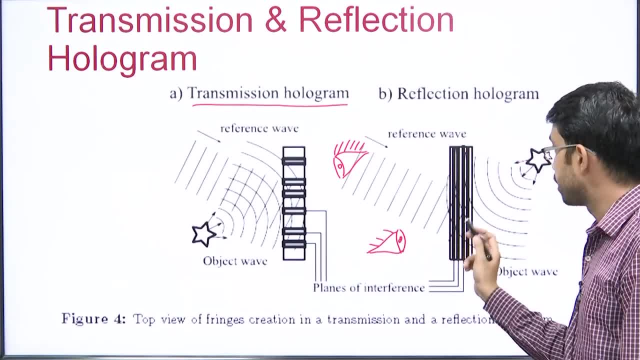 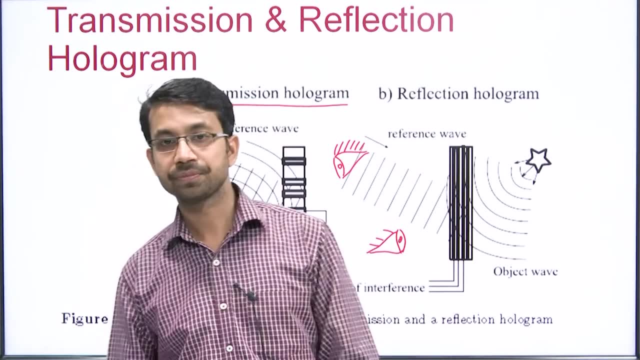 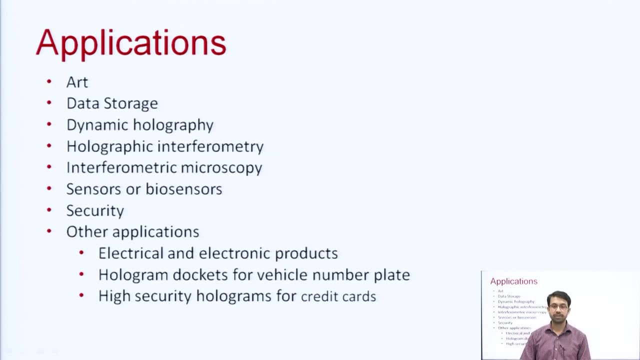 side of the reference beam. In this case, viewer is at the same side of the reference beam if he has to view the 3D image. ok, So this was about reflection and transmission holograms. Next we shall see some applications of holography Arts. it is used in entertainment. 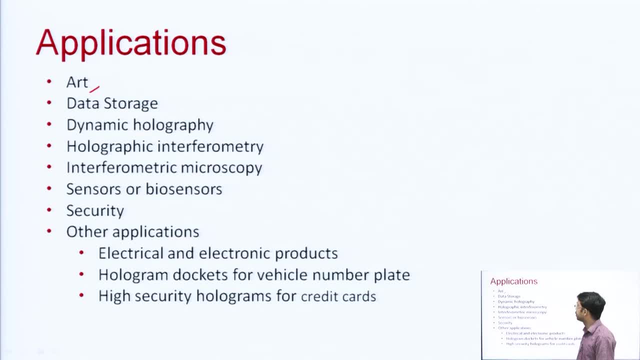 right for recording 3D images, 3D movies. It has a potential and it can be used for data storage. It can be used in dynamic holography. We shall see what is dynamic holography. It can be used at interferometry microscopy. It can also be used. it is used for designing. 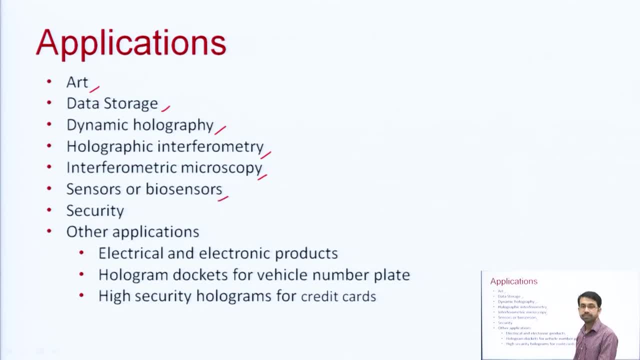 and developing sensors and biosensors. It can be used for security purpose. You can see every ATM card, every credit card and all the expensive products and even simple products like books. they put holograms on everything because it is not easy to record hologram. It is not easy to copy hologram. 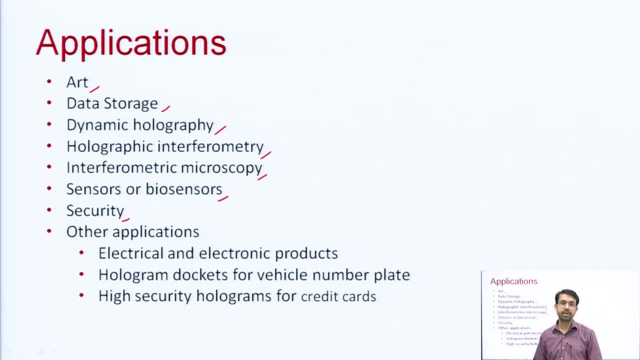 right. Hologram needs same 3D object from which it is recorded to record another hologram. It is not like you can copy a hologram from a from a hologram. ok, So for security purpose it holograms are used. Other applications are electrical and electronic products- hologram. 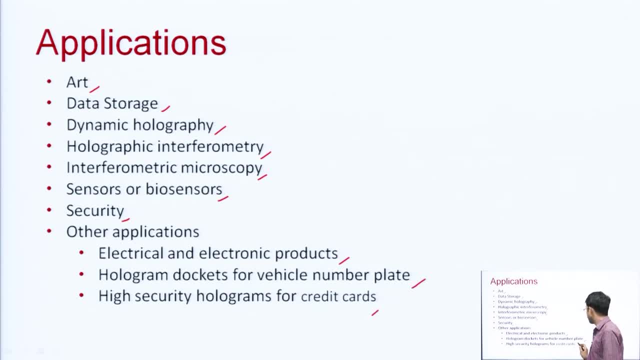 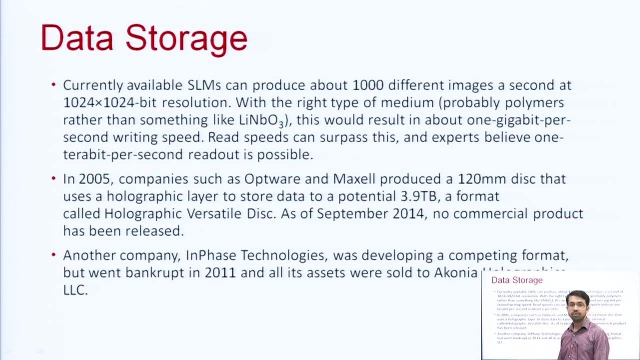 dockets for vehicle number plate. again, high security holograms for credit card, as we have already discussed. fine, Now, out of these, we shall discuss one application in details, that is, data storage. Currently, the holographic techniques that are available. they can. 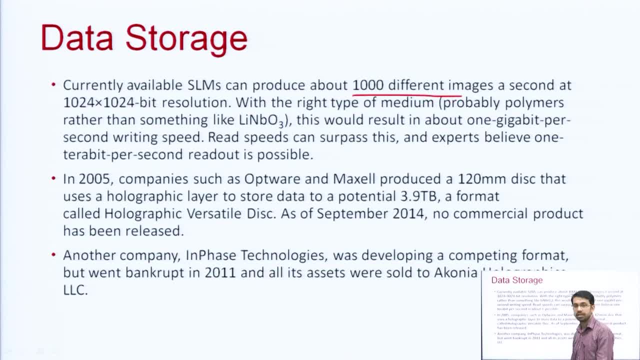 produce about 1000 different images per second. And with what resolution? 1024 into 1024 bit. resolution, that is 1 M, 1 Mega bit And 1, 1 megabit. how many 1000 images per second? So it is 1 gigabit per second with the right. 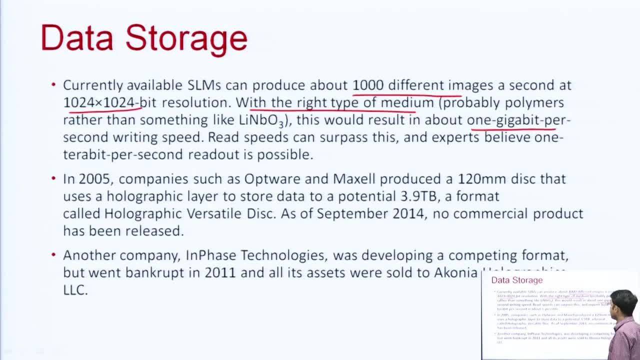 type of medium. this would result in about 1 gigabit per second writing speed. This is a very fast speed in comparison to currently that is available using semiconductor devices- 1 gigabit per second writing speed. reading speed is much higher And the speeds can surpass this, and experts believe 1 terabit per second readout is possible. 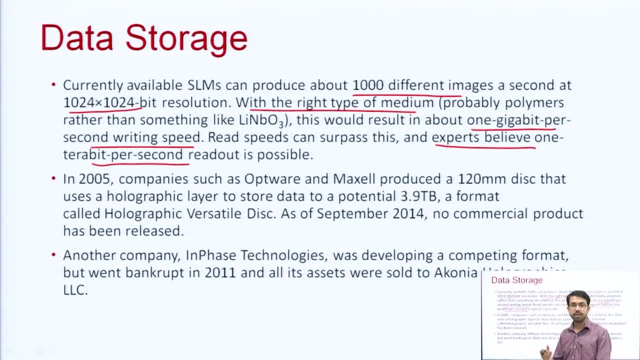 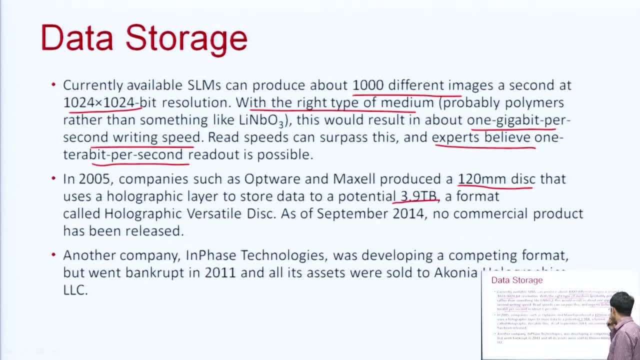 to store data. How much data? 3.9 terabytes. 3.9 terabytes on a single disk of 12 centimeter diameter. It was called holographic versatile disk, but it was not commercially available because readers are costly, writers are costly and disk is also costly. We need cost effective. 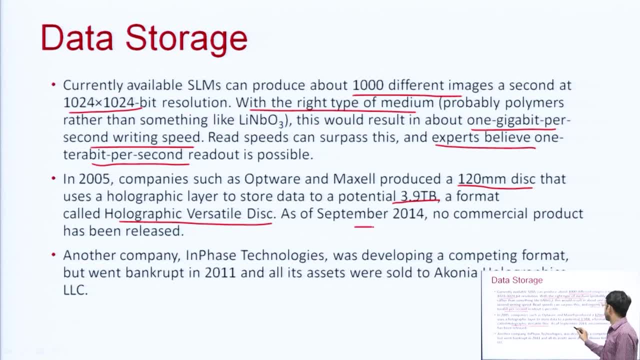 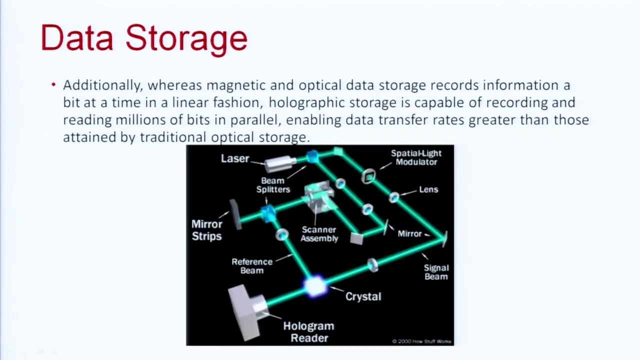 solutions Till September 2014,. no commercial product has been released. Another company that is named in phase technologies was developing a competing format, but it went bankrupt in 2011, and another company purchased all its assets with the name Aconia Graphics. ok, So this is a simple diagram that shows how a 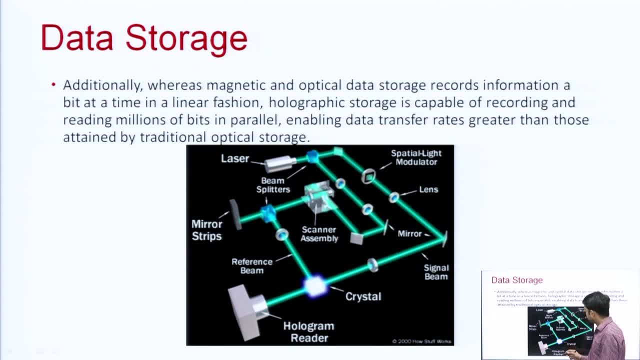 holographic system works, So holographic technology can be used to record data. So data will be recorded in form of holograms. This is the recording medium. it is a crystal, Whereas magnetic and optical data storage records information a bit at a time in a linear fashion. right They record. 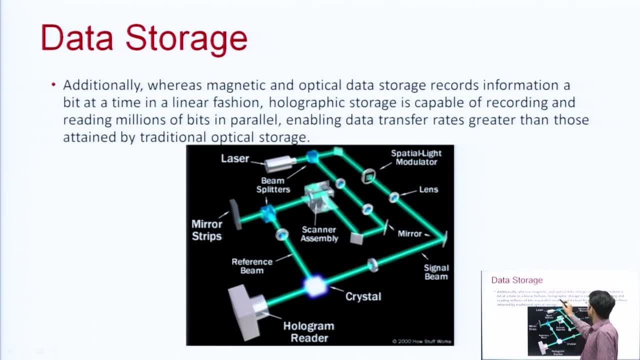 data in a linear fashion. Holographic storage is capable of recording and reading millions of bits in parallel. Millions of bits can be read parallely. and suppose if we have any processor that can process these millions of bits simultaneously, then it will be a very fast device enabling 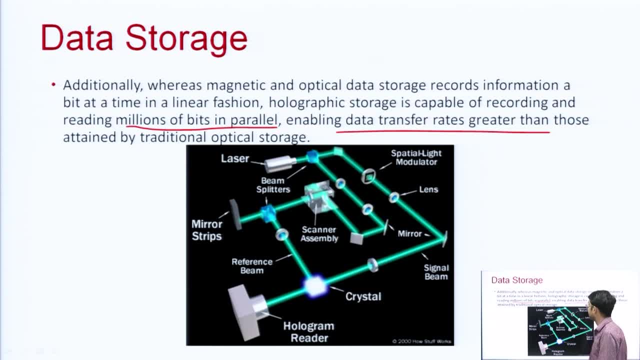 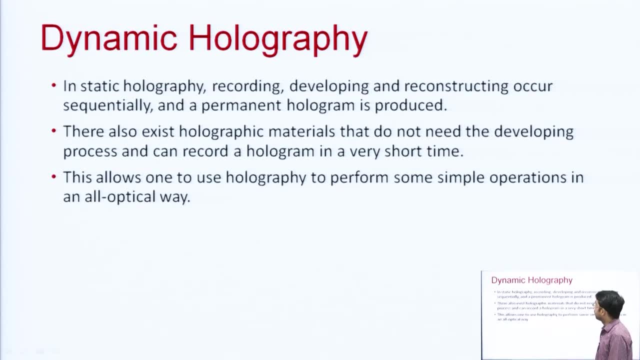 data transfer rates greater than those of traditional optical storage. ok, So dynamic holography, like recording a photograph and recording a video, So photographic scanning them. they do not require video recording. The thing they require is that they can also. 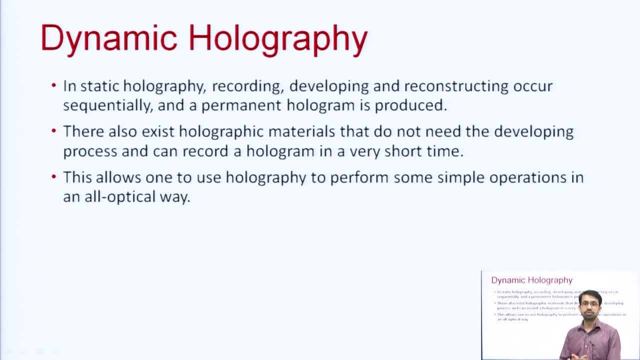 do the dynamic holographic record. So dynamic holography, like recording a photograph and recording a video, So photographic recording. so that is an important technical decision. A nice way to do a dynamic holography is to: So photograph recording is a static, video recording is dynamic, right. 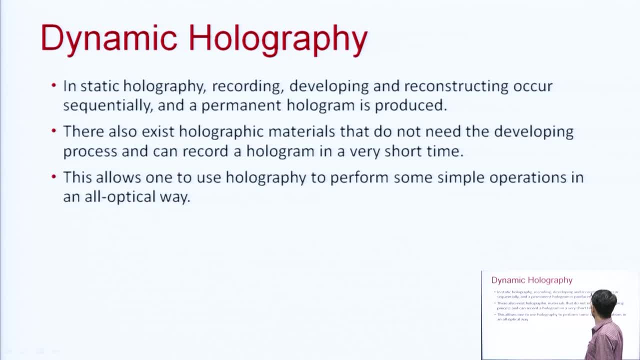 So in a static holography recording, developing and reconstructing occurs sequentially and a permanent hologram is recorded like a photographic film that was used earlier in old cameras. There we can also do this dynamically if we have correct materials. There also exist some holographic materials that do not need developing process and can 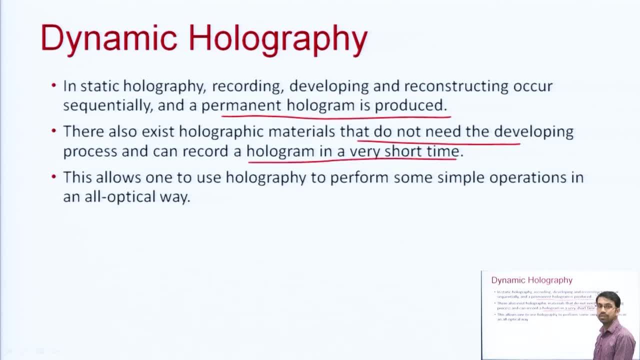 record a hologram in a very short time So we can use such materials for dynamic holography. This allows one to use holography to perform some simple operations in all optical way. ok, So all the operations- recording, processing- if all these can be performed in a dynamic. 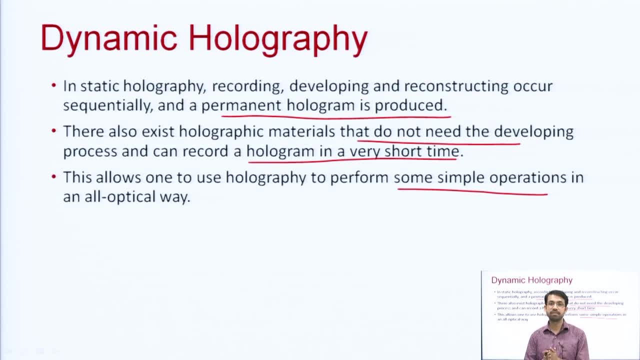 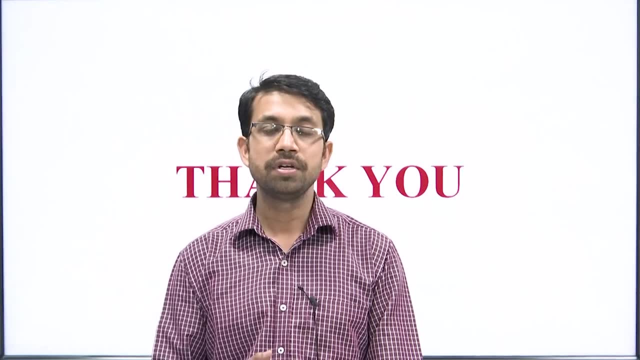 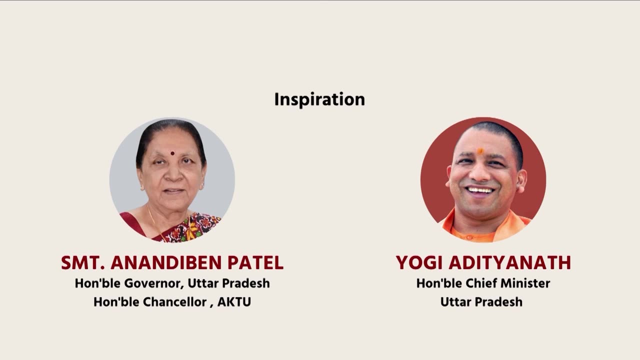 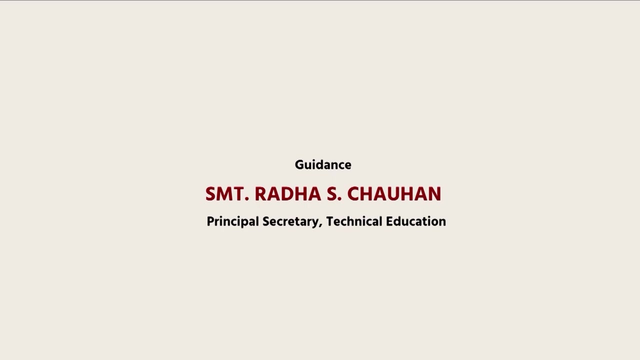 in a parallel way, then it will be very much beneficial. So these are the references. This was all about holography. In next lecture we shall discuss about optical fibers. Thank you.